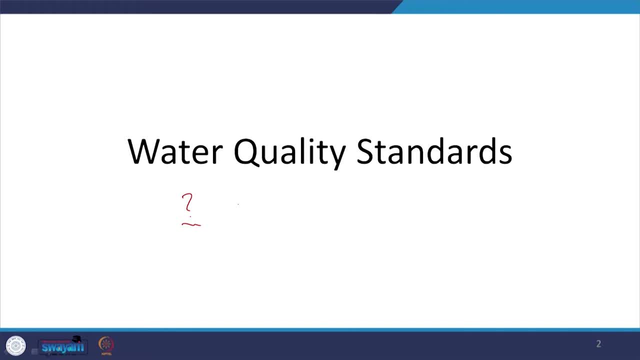 there is little to no disease transmission or pathogen transmission, So I am almost always concerned about pathogens. I am concerned about pathogens, So this is the most important aspect to keep in mind. There might be if I am using groundwater, there might be deposits or contamination of 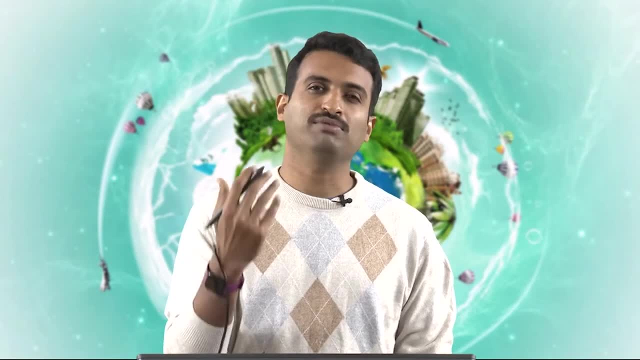 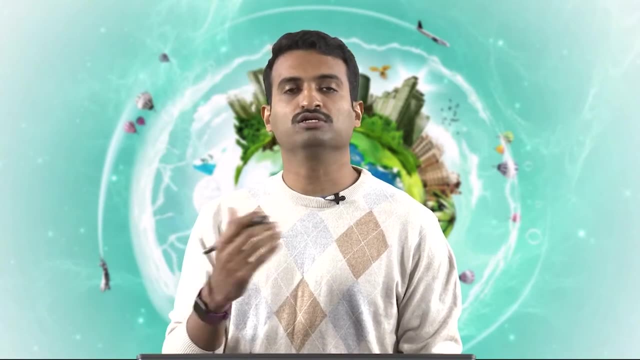 groundwater due to various sources. So maybe then I need to look at a particular treatment mechanism for that particular kind of toxic compound. But in this course we are going to look at the general aspects. So after the pathogens we will look at 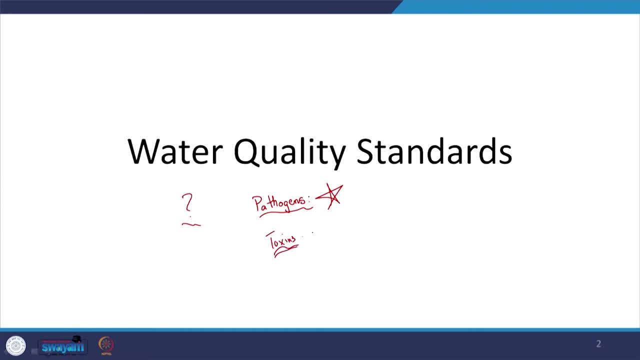 toxin, toxins or such, But typically relatively rare cases, So we will not go into that now. Another aspect that we typically almost always consider is total dissolved solids and total suspended solids. So these are indirect indicators. So that is the relevant issue. 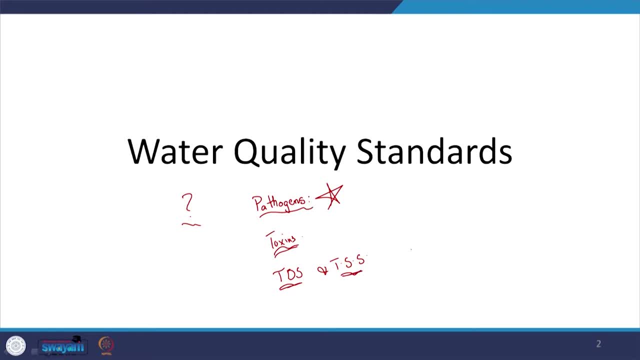 As you know, total dissolved and total suspended solids. the sum will be equal to the total solids. Total suspended solids will give me an idea about pathogens and quality of water, But it is not a direct correlation but it will give me a pretty good. 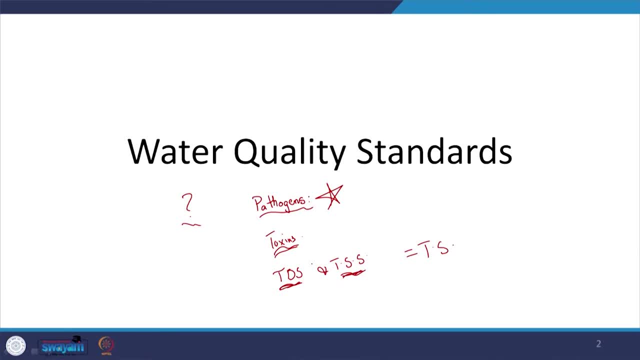 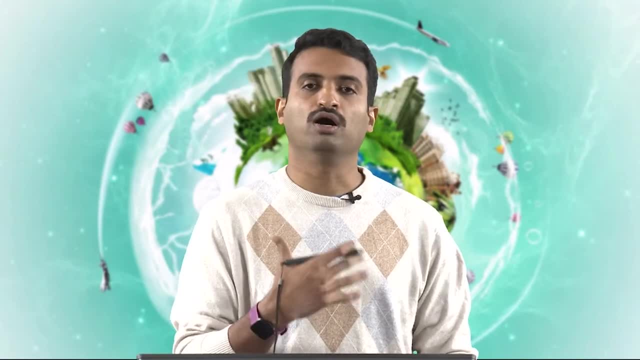 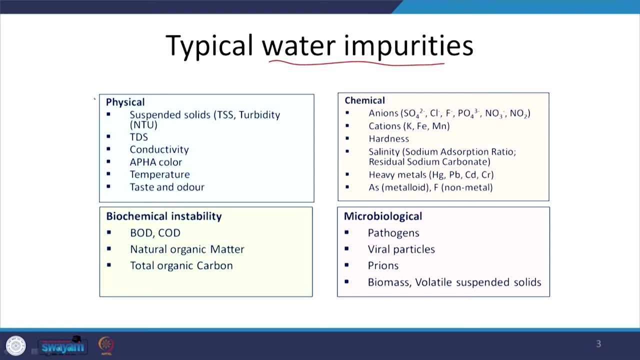 idea And dissolved solids will give me an idea about how much or how many ions are such there are in that particular water. Too high, difficult, too low, not fit for consumption? Let us move on and look at the relevant aspects. So typically, when we talk about water impurities, 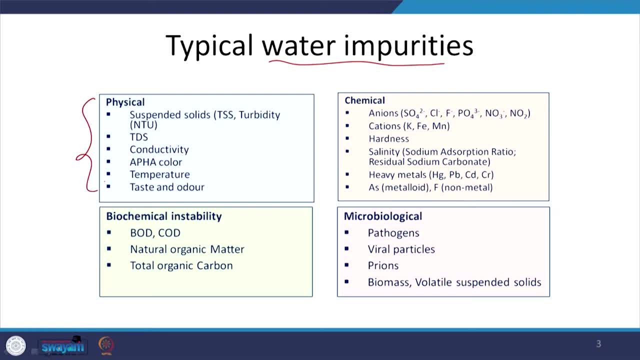 we look at physical parameters to be able to estimate this water or water impurities, and then chemical, And then we will also look at it later. So this is the general analysis and then we will, and biochemical and then microbiological parameters In the context of wastewater. 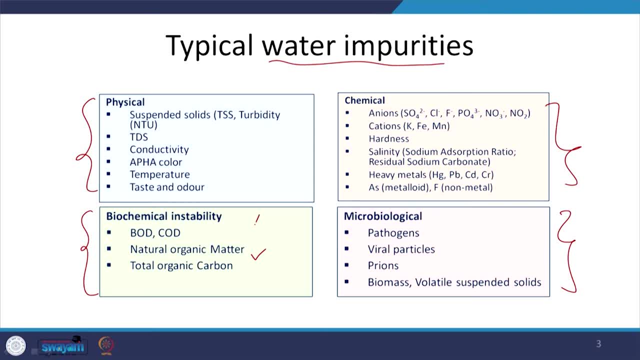 we looked at these, but in the context of water or drinking water, we will not look at this. We will not look at this. What do we typically look at? We look at the physical, chemical and microbiological parameters. Total suspended solids: we looked at that. 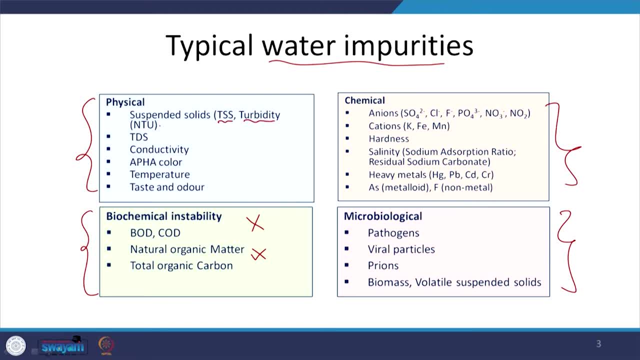 How do we measure that? That is, using the turbidity meter, and the units are NTU, TDS, total dissolved solids, and we can measure that by conductivity or by direct measurement. We look at the color of the water temperature too. For taste and order, there are some tests. 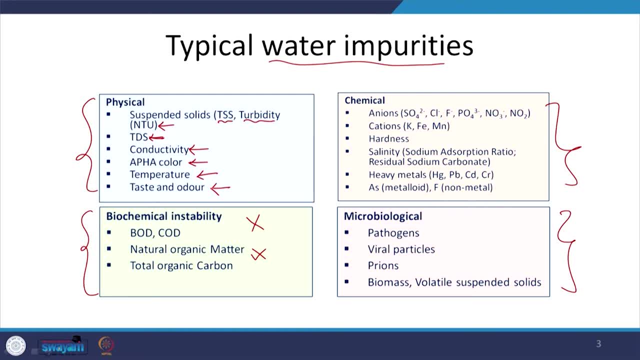 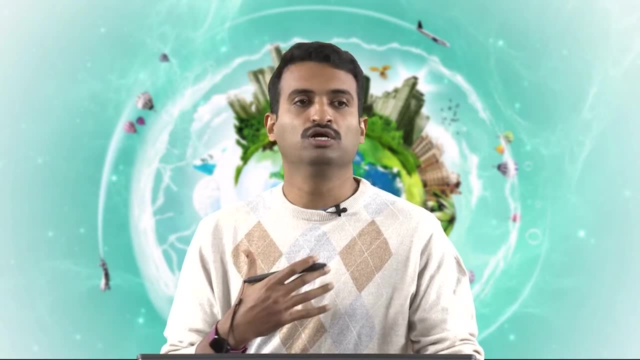 but in India typically, if it is not objectionable, that is good enough for us. When we talk about chemicals we look at the usual cations and anions Here, anions negatively charged that will, at higher concentrations, lead us to have some diarrheal issues or digestive issues or maybe pain in the joints. 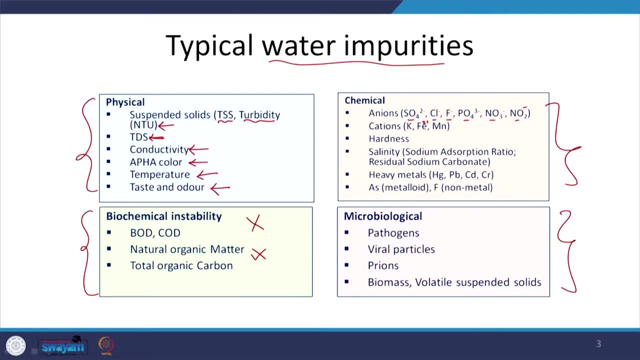 We have those some cations- Fe2+, Mn2+ cations- positively charged. This is 2+. if it is not clear 2+, Then hardness, because if the water is too hard, meaning I have too high a concentration of calcium or magnesium. the bivalent cations: 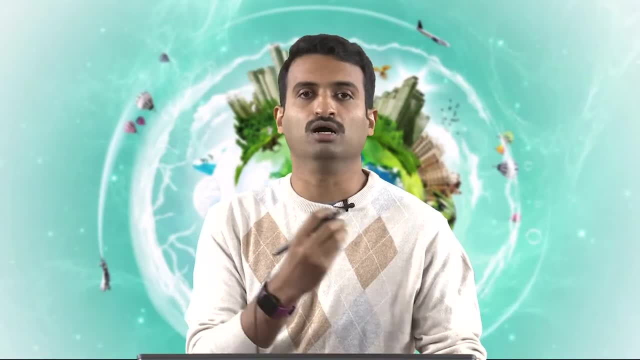 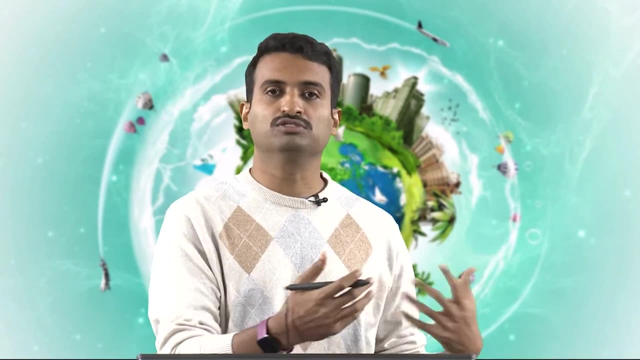 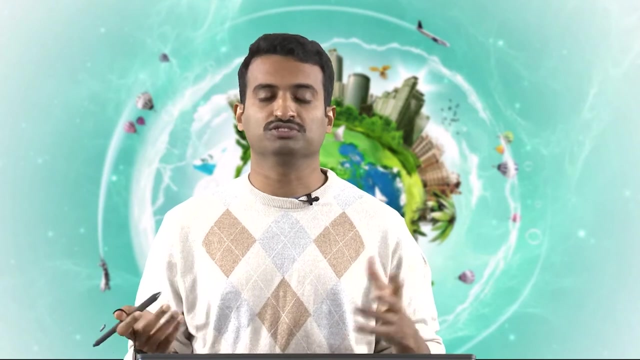 that will not let my surfactant or soap form the relevant leather, And I will have issues whenever I am trying to clean my utensils or clean myself or the clothes, And also it can lead to scaling of the relevant pipes or utensils and such. 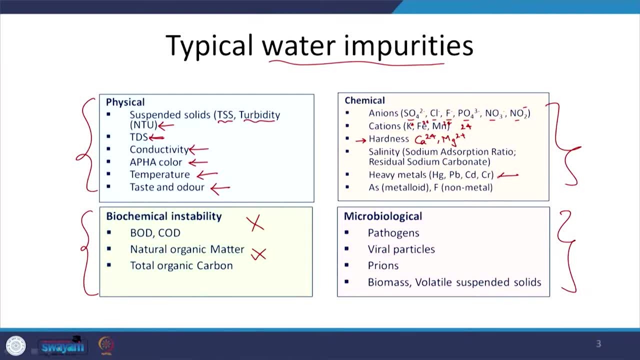 That is an issue. And heavy metals, which can lead to toxicity, arsenic and fluorosis too, due to fluoride, But we are not going into detail. Now the microbiological: we have pathogens and typically viral particles, but viruses in general come under the category of pathogens. Typically we are concerned with microbiological. 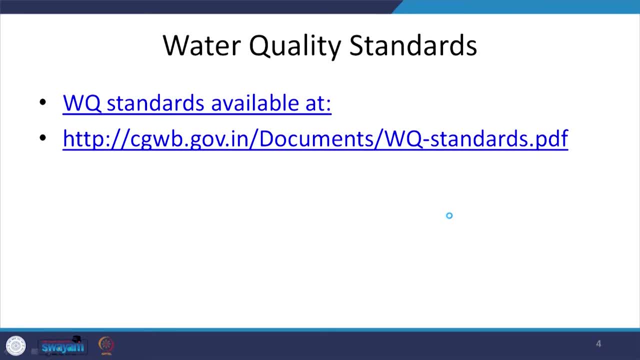 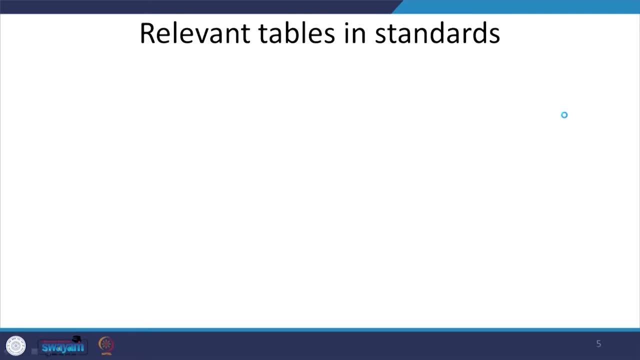 parameters too. Let us look at where I can get this data. There are different sources. One is this particular link that you can copy paste and look at Relevant tables in standards. I am going to look at the standard, but let us look at the general classifications. 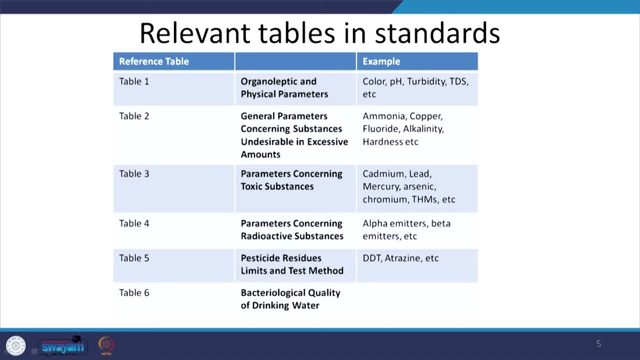 Our characterization. First one is organoleptic and physical parameters, The general parameters which we discuss, which we measure when we talk about water or water quality. Then the parameters which, when excessive, will have undesirable effects. Copper will also have toxicity. that will come there also in toxic substances. Typically I am concerned about hardness, alkalinity, ammonia, iron and so on and so forth. And then we need typical metabolic substance, that is, admit that ahead of the two processes, cuyt is amyl folate and one foodう chocolate. This is another part when we are considering the matter of quality, pathetic factories. 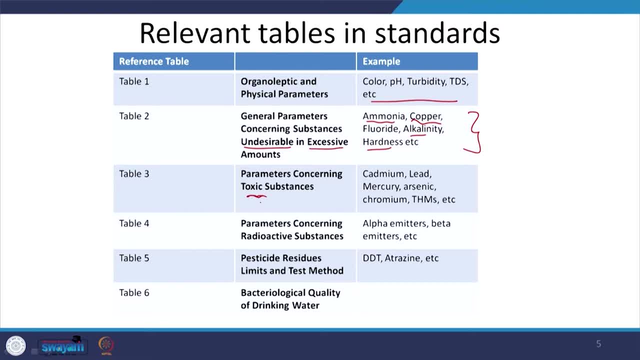 There are some Pifashioned, while it is seen as terrible. You may think of litchi, avant-garde recherche, let people think of these places, but that is not the case. So uh n lenan. Table 3, about toxic substances, heavy metals, typically cadmium, lead trihalomethanes, which 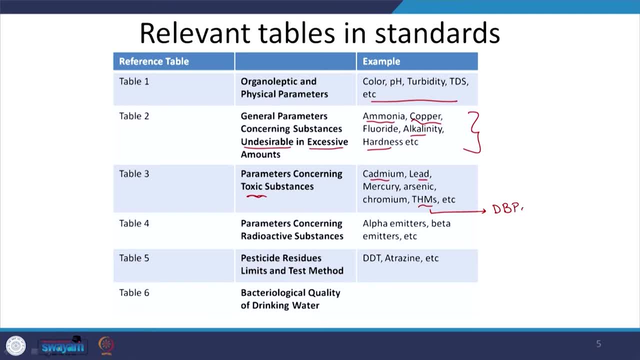 are the disinfection byproducts we already discussed and so on and so forth, And radioactive substances, but rarely do we measure this in drinking water because, okay, for example, I know, I think there is a student group here in IIT, Roorkee, Unad Bharat Abhiyan. 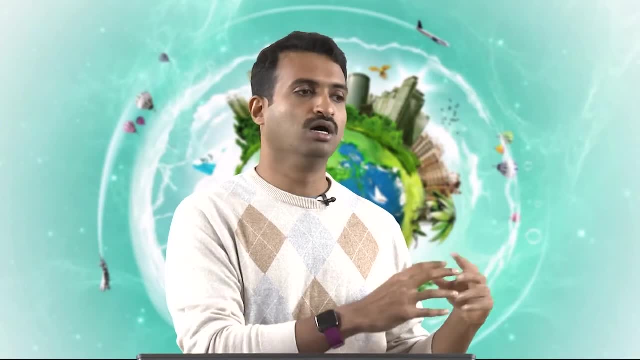 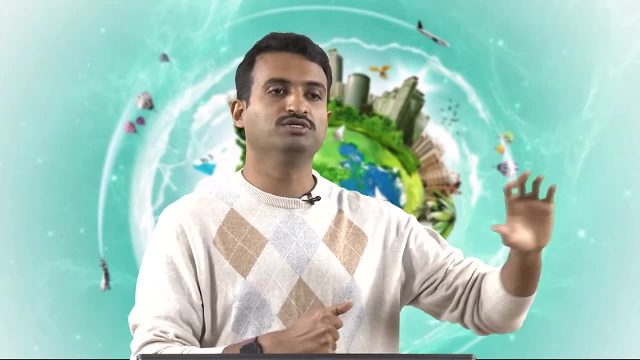 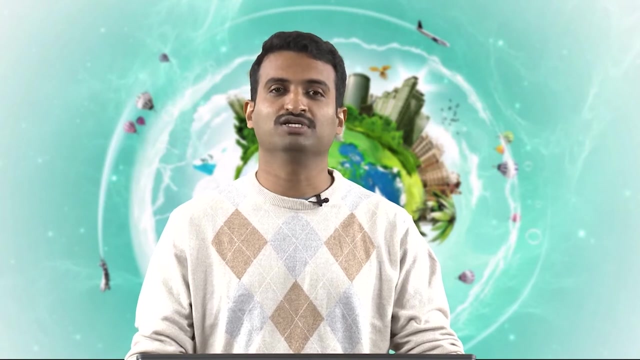 they were trying to look at the water quality of a particular village or the water from the quality of the groundwater that is being consumed by villages nearby. So they say, Banu, get the test done. okay, I say for what parameters? So then obviously they are not sure because, as you see, when we say get the test done, 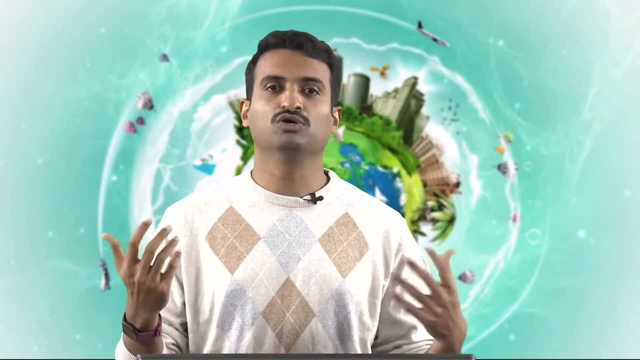 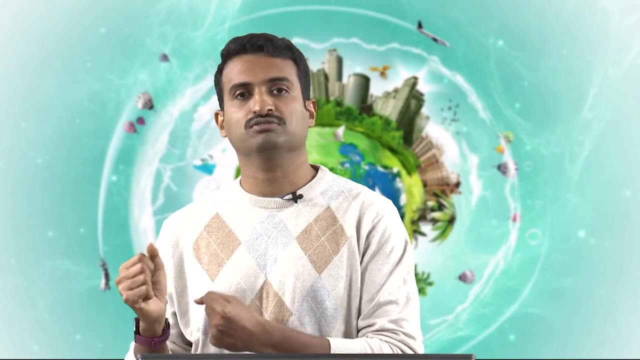 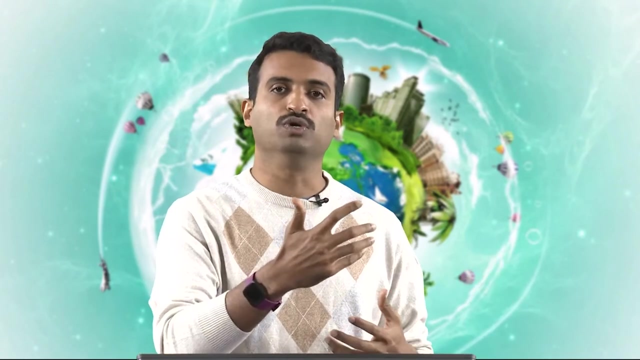 there are quite a few parameters. again, we will look at the table. So if they are looking for a specific adverse effect, we can try to you know, understand the cause and then look for those. If not, the usual water quality test will not be exhaustive. it will look at only a. 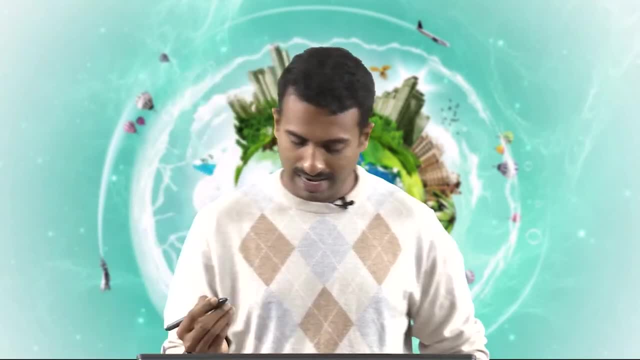 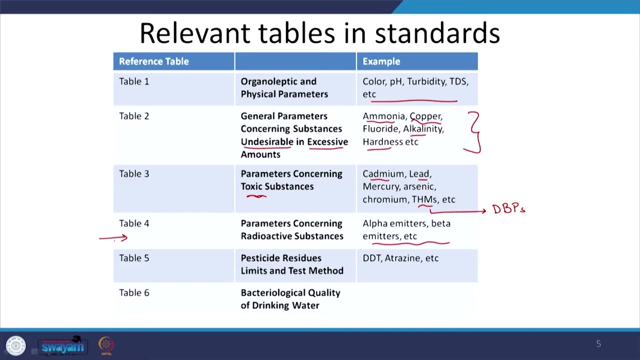 few aspects or such. So that is something to keep in mind And obviously, as I mentioned, rarely do we look at radioactive substances, But if there are, you know, relevant side effects or such maybe, then we will have to look at the radioactive substances. 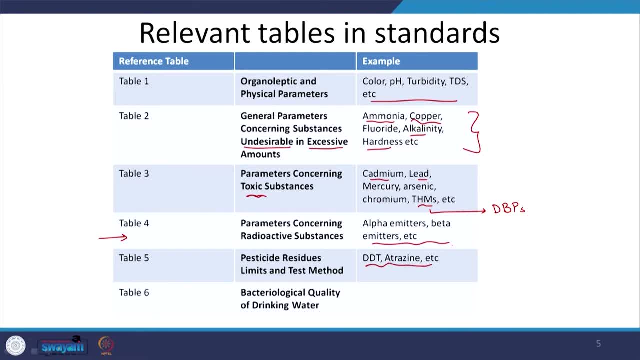 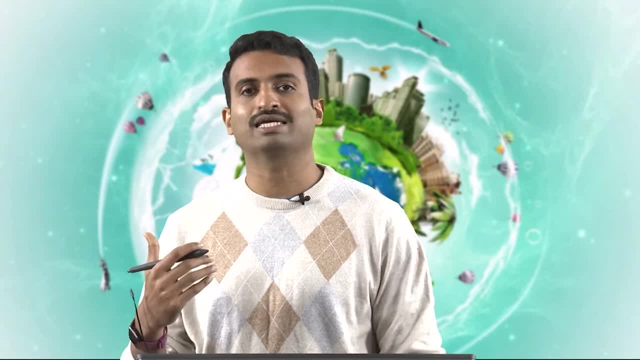 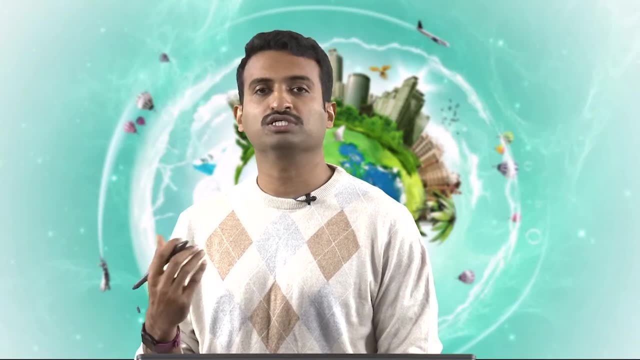 And again similarly DDT and atrazine. if you know, you suspect contamination or you see issues with respect to fertility or lab Lack of fertility or increase in infertility levels or decrease in fertility levels, typically that is due to pesticides And you have different neurological issues too, due to pesticide consumption, even in. 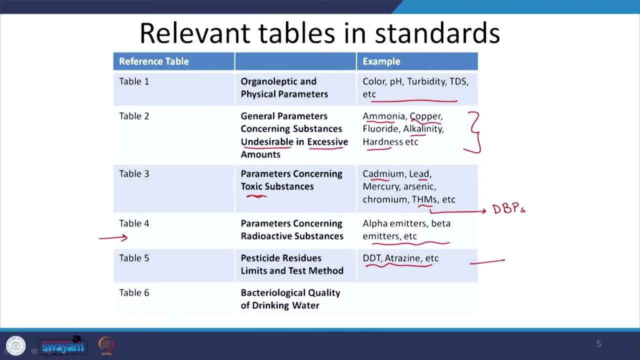 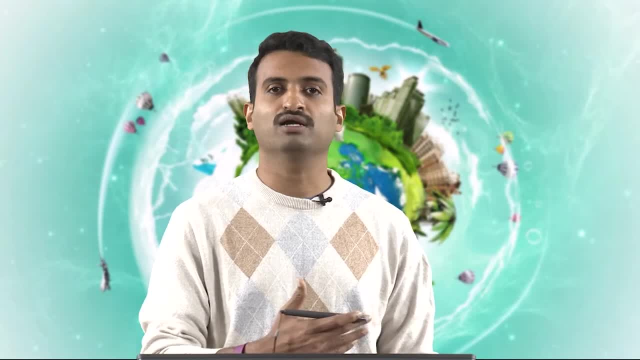 low concentrations over time, then we will look at it. But if you say, hey, man, get the water quality test done, you know, at the usual price of, let us say, 3000 rupees or so per sample. I cannot, or one cannot, measure all the samples. 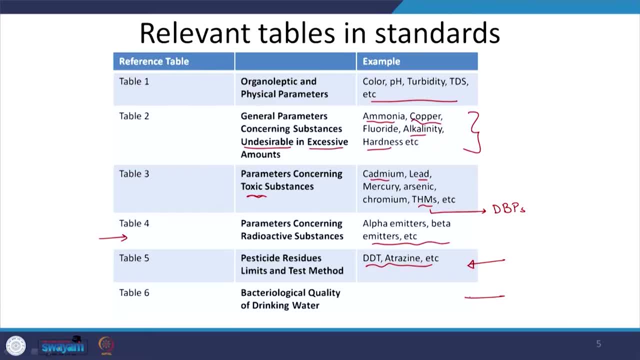 that is something to keep in mind, But obviously we will always measure all the samples. So that is something to keep in mind, But obviously we will always measure all the samples Or try to understand the bacteriological quality of drinking water. 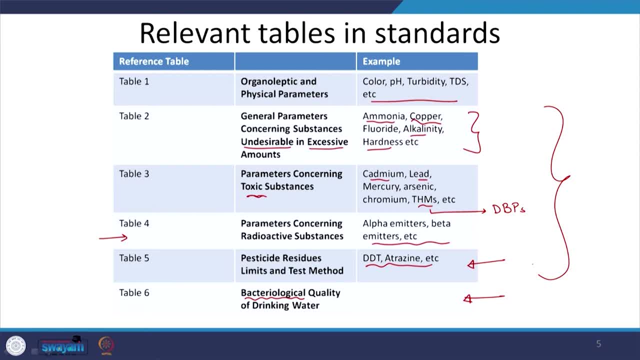 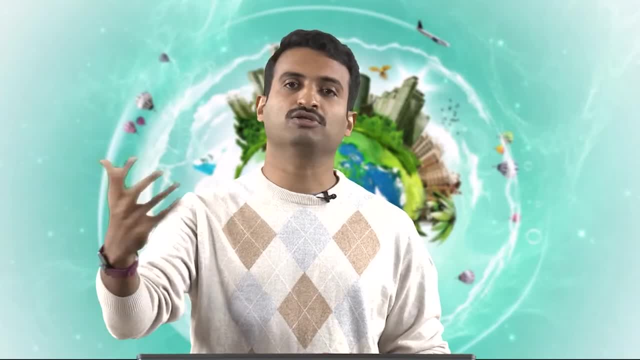 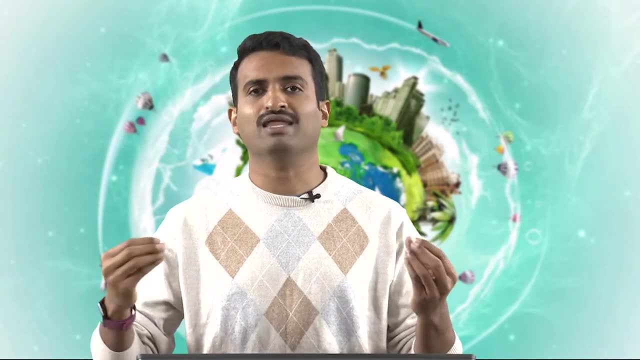 All this will typically have long term issues, as in: I keep drinking this water over a period of time, Unless the concentration is so high due to, let us say, some accident or spill. let us say radioactive substance or arsenic came into the picture at very high concentrations. 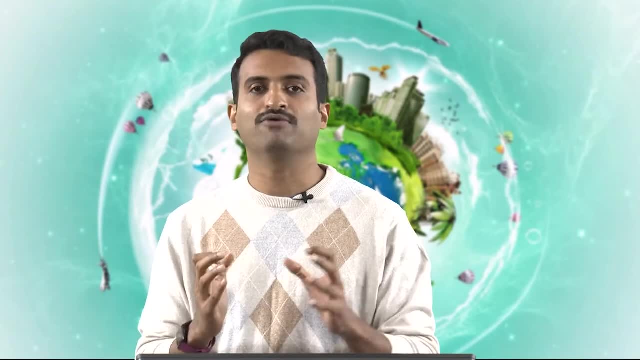 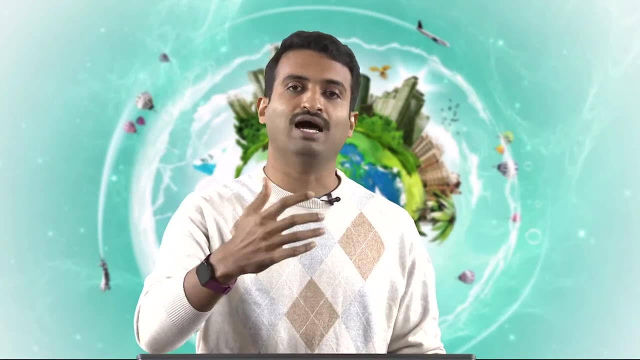 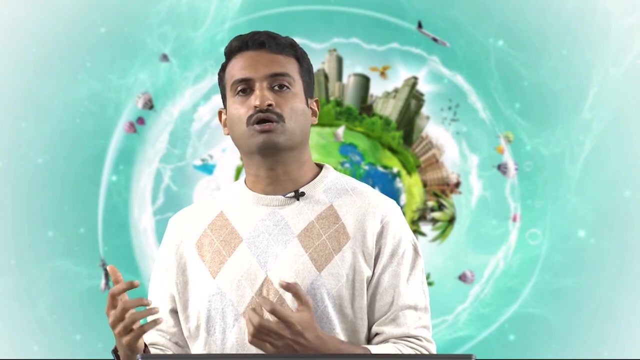 then I might have acute or short term effects, But in general I will always have what we say or I am always concerned with these bacteria biological effects, because they will always have, almost always have immediate effects And, as we know, death due to diarrhea is one of the major cause of death among the infant. 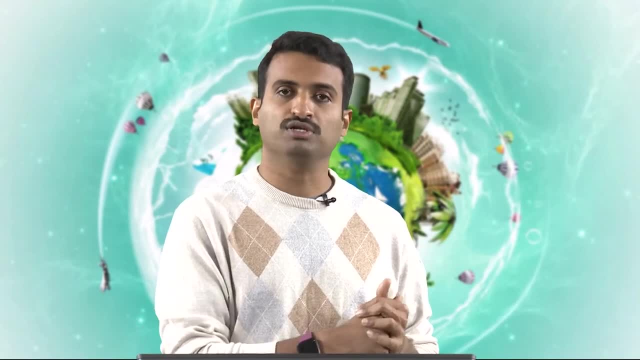 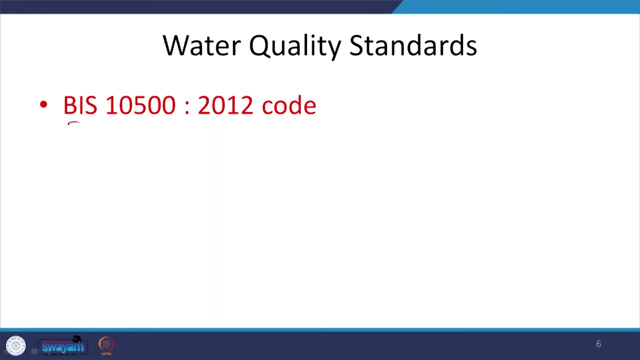 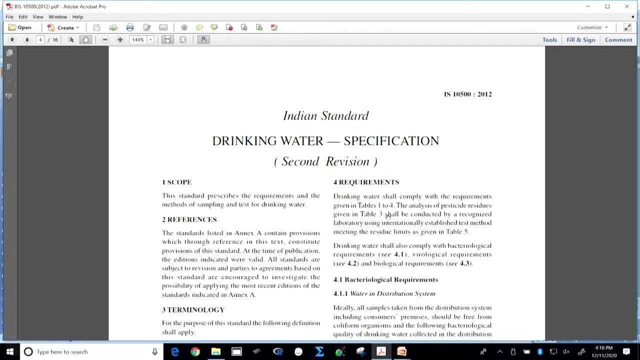 and the more susceptible population, which is the children. So that is something we need to be remarkably concerned about in India. So let us look at the relevant code: BIS1050020112 code, I guess, right. Okay, So what do we have here? 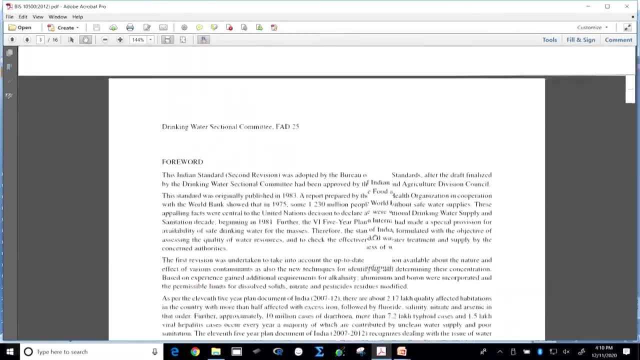 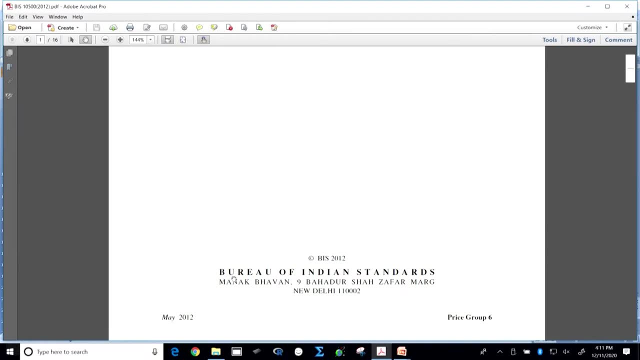 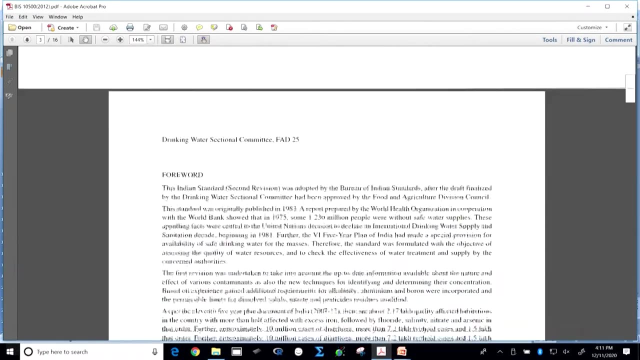 The second revision and such all. this is fine. Okay, drinking water source. okay, this is Bureau of Indian Standards, I guess? okay, Bureau of Indian Standards, And we already looked at the link earlier. this is the revision. So from time to time they revise and update based on the best available practices, and 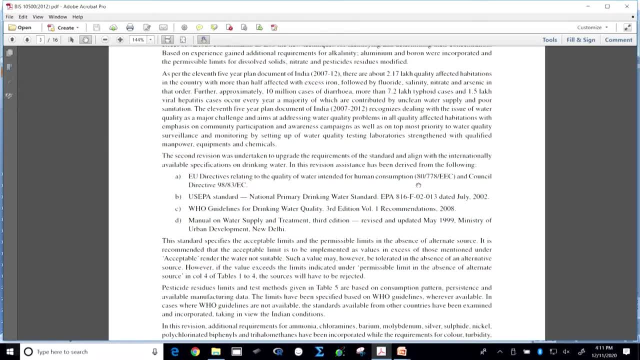 technology and needs to keep in mind that they also looked at the EU directives, US EPA, So it is more or less based on what we observe in India and also what the other developed countries are doing or have done. they typically have more stringent standards, but we cannot. 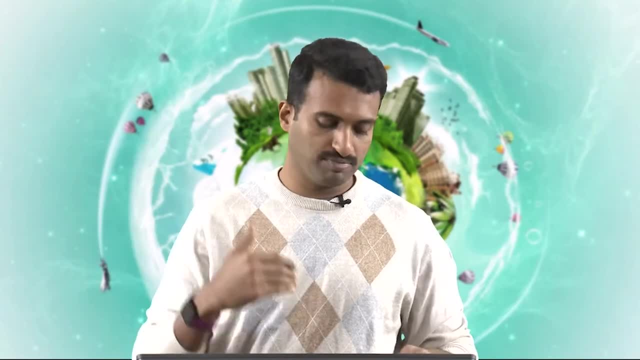 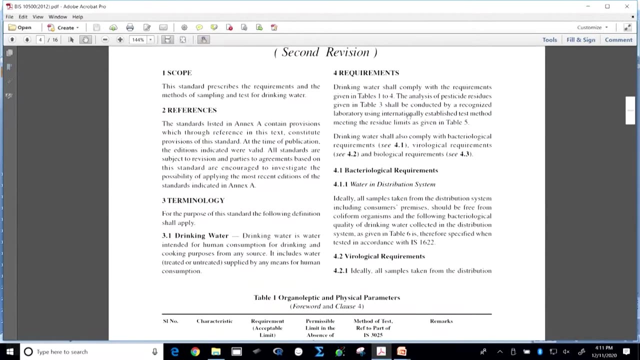 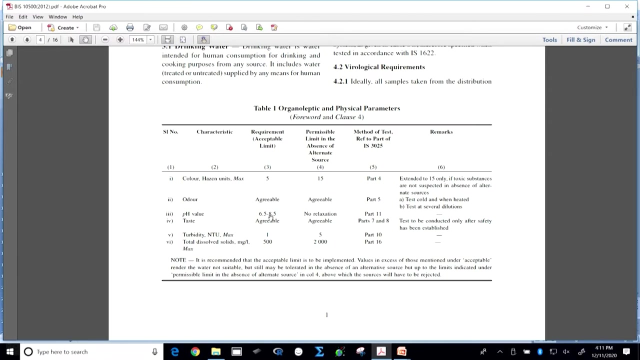 aim to achieve those standards right away, But it is a step towards those standards, yes, and World Health Organization guidelines. So, drinking water, as we mentioned, different kinds of parameters, The first one, the generic parameters, so pH 6.5 to 8.5, taste agreeable, but no specific. 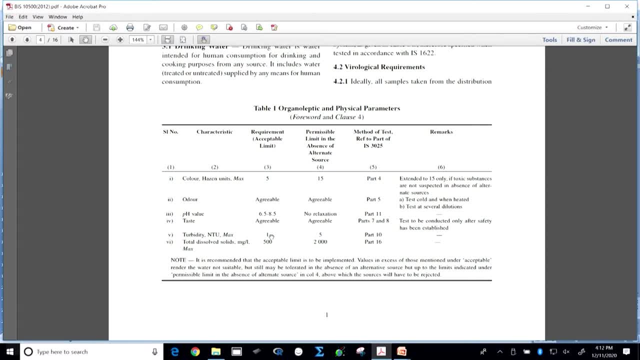 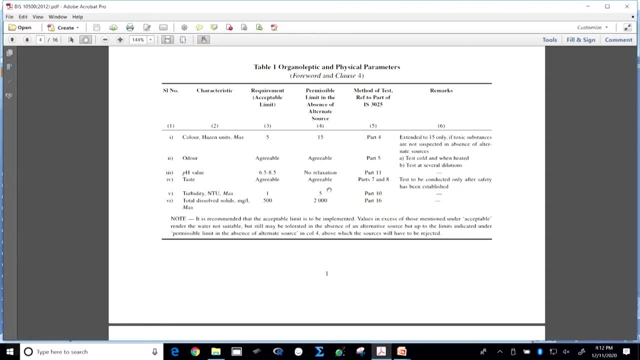 test turbidity- pretty much important. we have to measure this one and certainly less than five total dissolved solids 500 and 2000,. one aspect I would like to mention here: So quite a few people now in India have these household water purification devices. right? 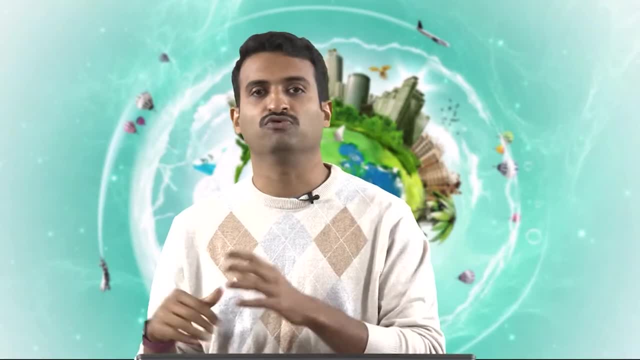 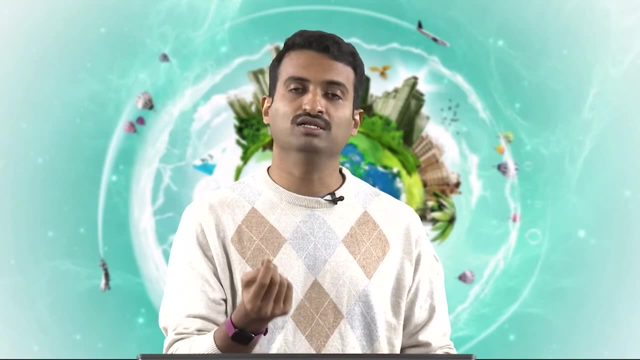 different companies: Aqua Life, Aqua Pure Water Guard, so on and so forth. Nobody typically tries to sell you this RO unit. the RO will have- or you know, the effluent from RO will have- very little dissolved solids, not zero, but maybe 10, or maybe 20,, depending. 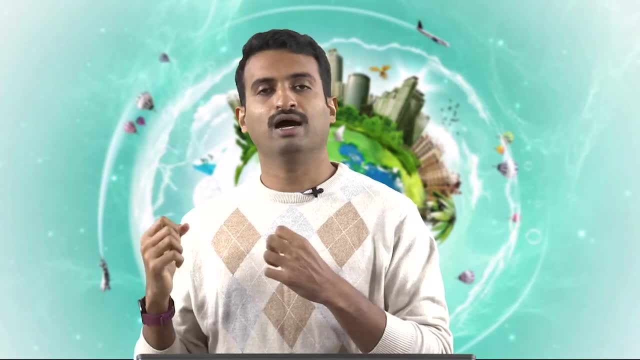 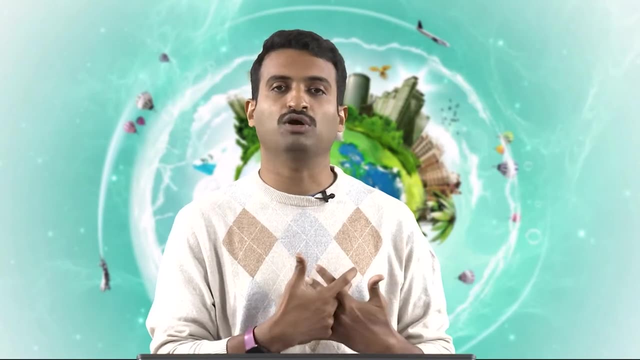 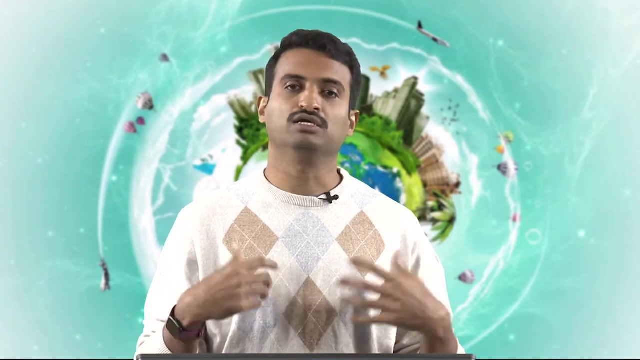 on how well it is working or such right. And here the issue is that if I drink water that has only 10 or 20, what do we say dissolved solids? that is not at all good for my health And it even has effects on the cardiovascular system, right and digestive system and such. 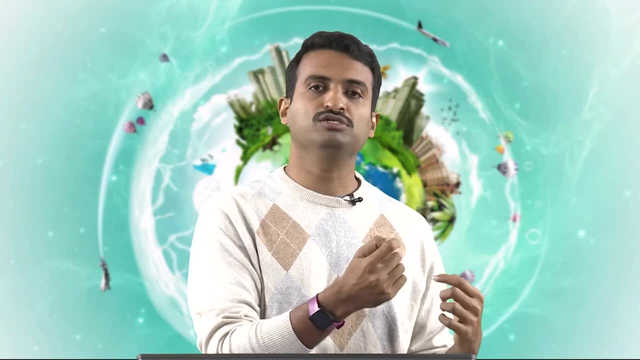 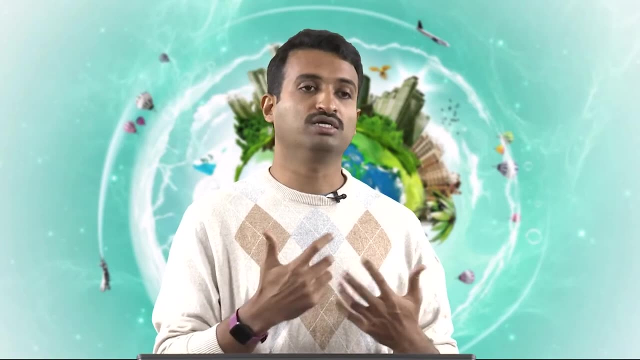 too. Again, I need all these ions, fluoride, calcium, magnesium and such- in little quantities. my body needs that. Without it, again, I will have what do we say? issues, different issues over the time. So just saying that: okay, RO, and get that done, you know, as a solution for everything. 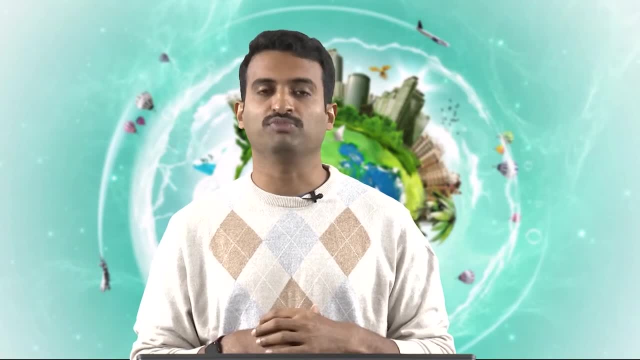 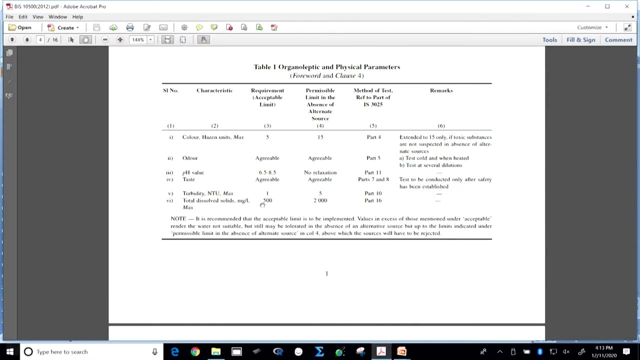 that is misnomer, if I may say so. so that is something to keep in mind. In general, the required or acceptable limit is 500, but 300 or 350 is what is fine, or 300 milligram per litre. About that you will see. 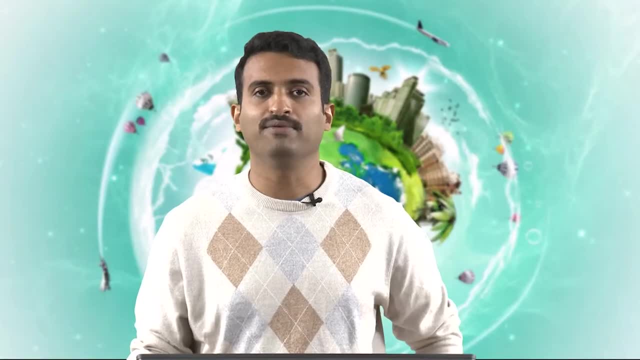 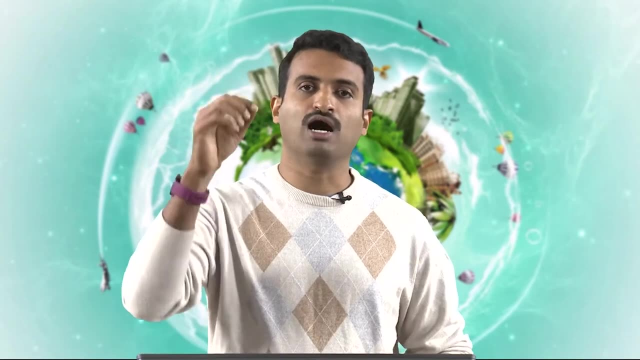 You will start to feel some discomfort, depending on where you have been living and how long you have been. what do we say? consuming that water, For example? typically people will say RO, but what is the? what do we say? the person? 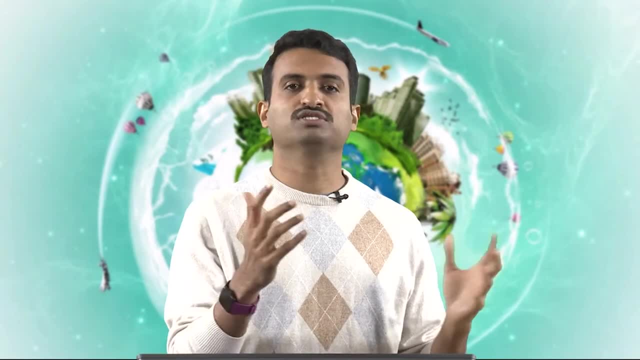 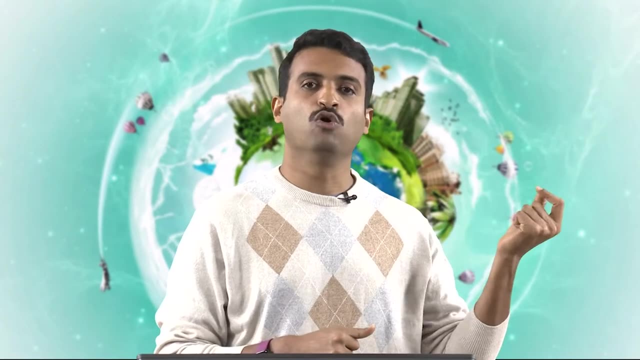 coming to your home to install that RO unit. he will ask: what is the TDS that you want? So, okay, you can say 300, right, so that is one way. but he does not set the settings such that the water through the RO unit will come to 300, what he will do is he will bypass. 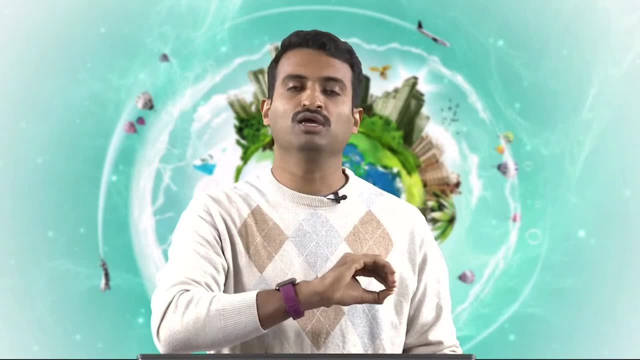 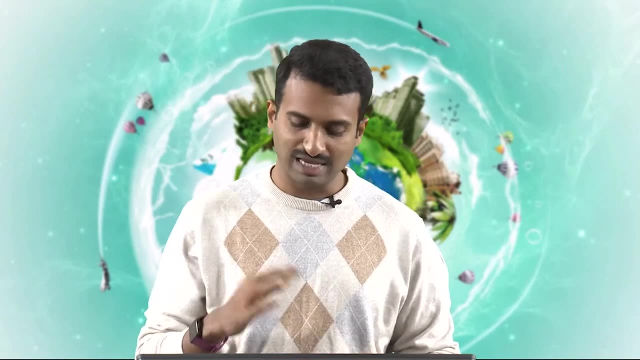 some water, But some of the water will not go through the RO unit and mix some of the water coming through the RO unit, So that the final of these two streams will be around 300,. again, we will look at these aspects later. 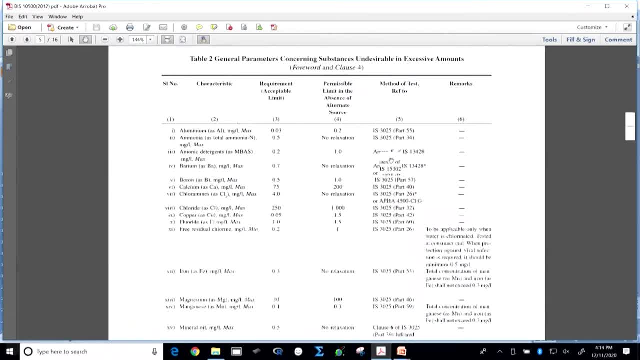 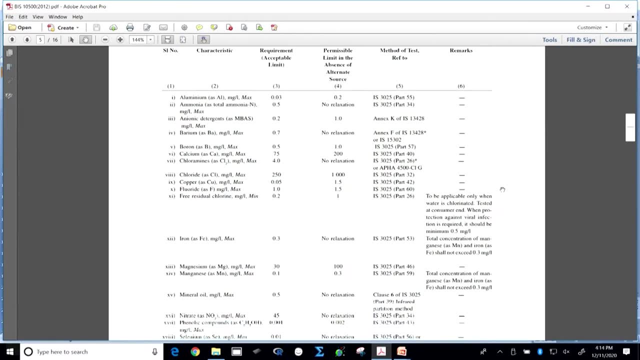 So organoleptic and physical parameters, right, and then the general parameters concerning substances which are undesirable in excessive amount. this is something we looked at earlier, And one other aspect I would like to mention is that we also have the kind of test as in. 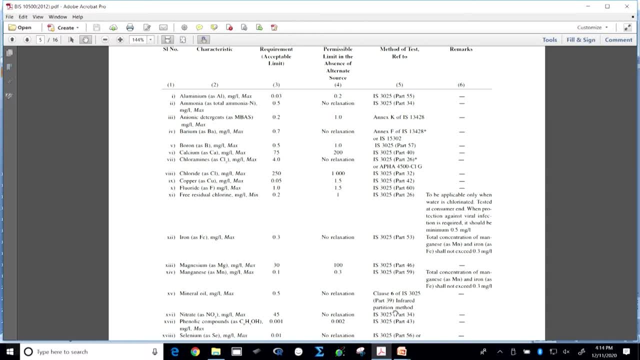 if and when. So there is- what do we say? doubt or confusion regarding the authenticity of the tests or quality of tests. So you have the relevant method and the reference that is given out here. So, as you see here, aluminium, ammonia, barium, boron- but rarely would you see boron in typical. 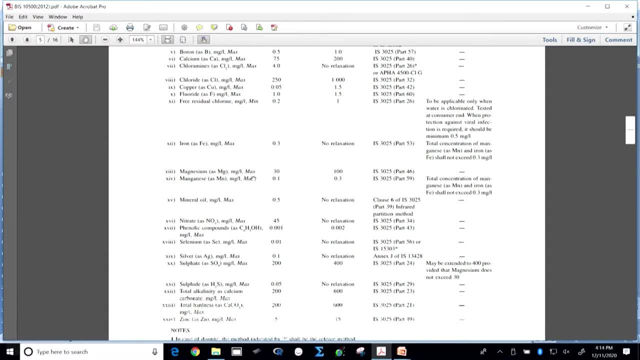 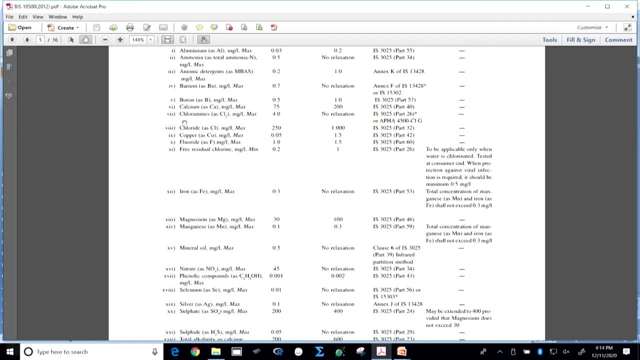 waters, chloramines again rarely. but if you have a wastewater that has been chlorinating there, what do we say effluent? and you are drawing water from near that particular discharge point, I mean the bitumens will be a factor. 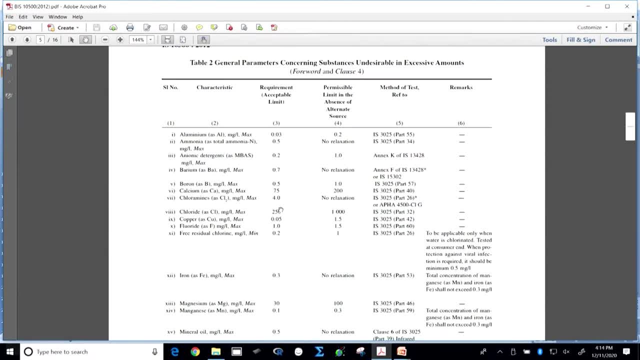 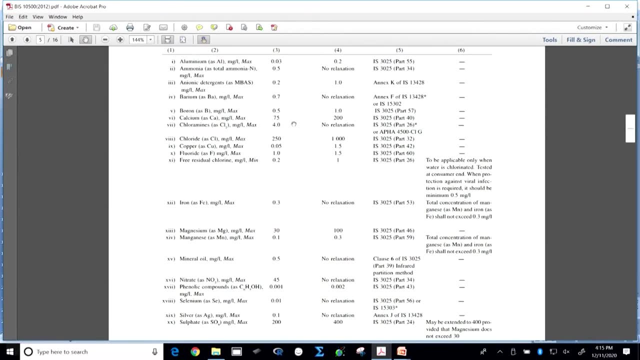 Chloride? yes, you will have it. So that is why the acceptable limit is given as 250 milligrams per liter. as you see, it is pretty high. It is not pretty. what do we say? it is not toxic or undesirable, even at relatively high. 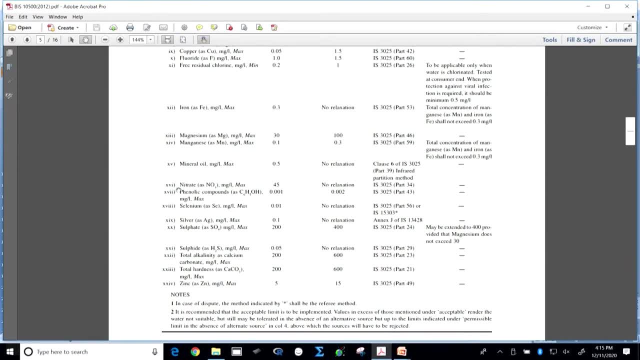 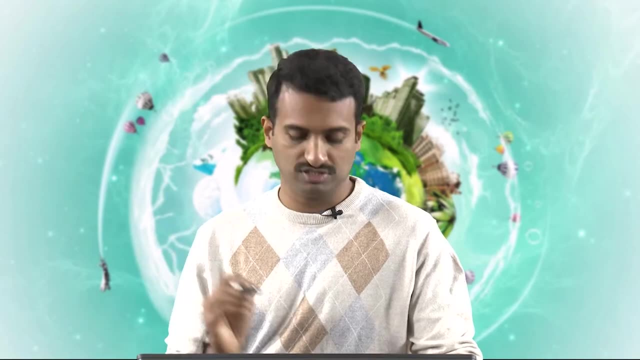 concentrations And then you can see the relevant standard. So nitrates- this is something that we mentioned or discussed in the context of our wastewater, that high nitrates are not good for. what do we say Drinking water, especially for or in the context of the infants they will, or their ability to transport. 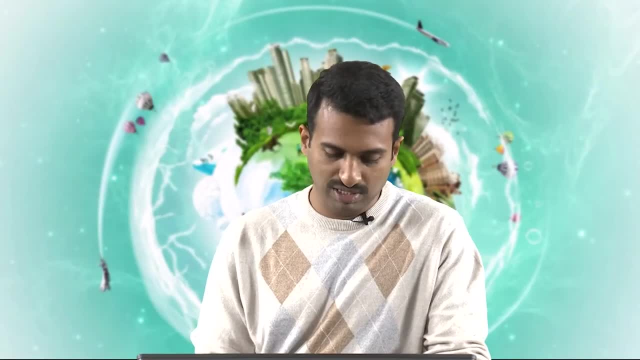 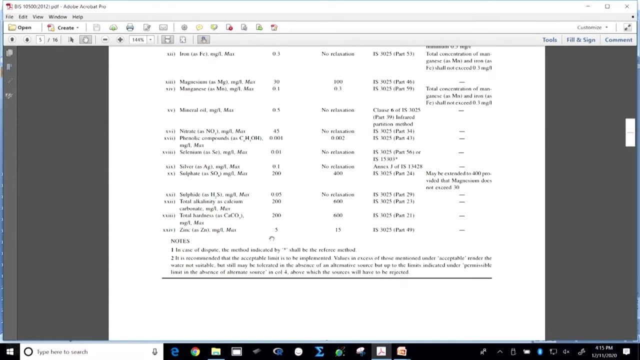 oxygenated blood to different parts of the body will be remarkably effective. This is something we discussed earlier and that is what I want to point out here: Calcium, hardness and such 200, and so on and so forth. Then we will move on to the toxic. 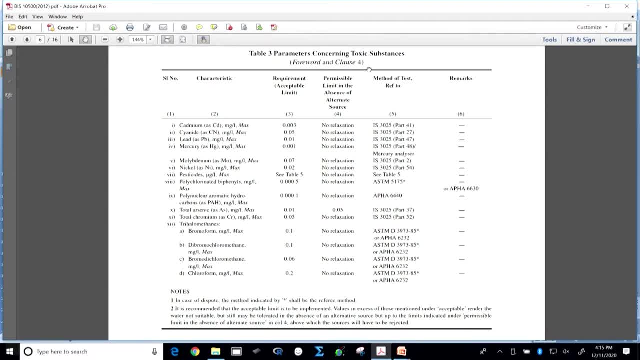 substances which will have either carcinogenic or toxic non-carcinogenic effects. Some compounds can lead to cancer and also other non-carcinogenic effects. That is something to keep in mind: Cadmium, cyanide and such. I am surprised arsenic is not here. They would have probably classified. 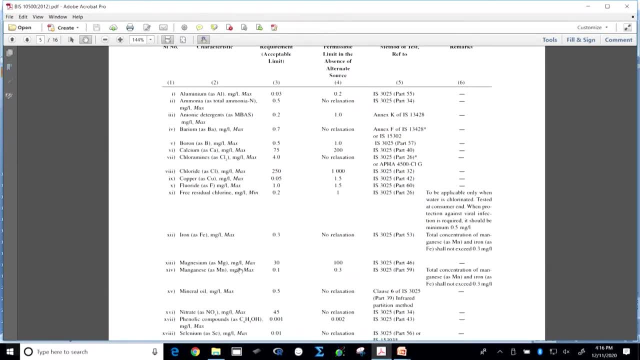 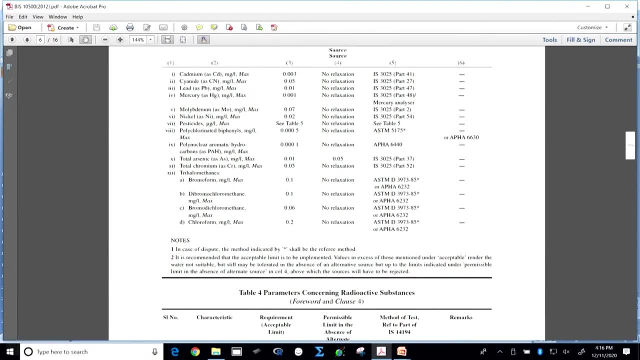 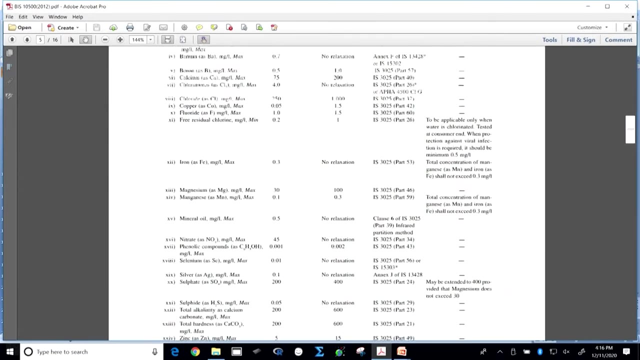 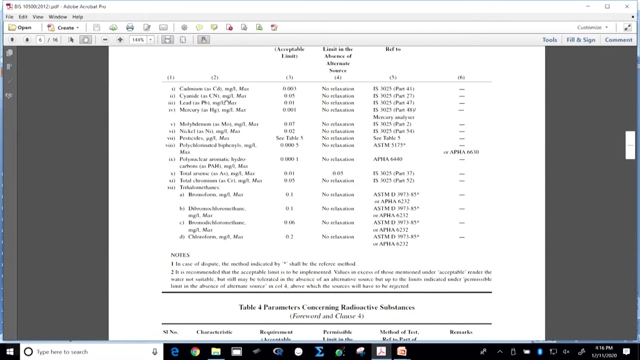 that here. That is another surprise. I am surprised arsenic is not mentioned, because that is a considerable issue, in India at least. Maybe it should be in one of the parameters somewhere, but probably I am unable to find that out. You can look that up. It should have arsenic somewhere or the other. Let me move on Here. you 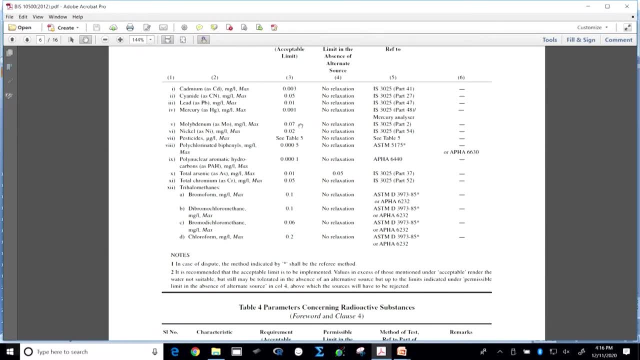 have the toxic compounds or relatively more toxic compounds. That is why you see that the acceptable limit is much, much lesser. here We talked about the disinfection by-products. That is why we see the trihalomethanes, which are one class of disinfection. 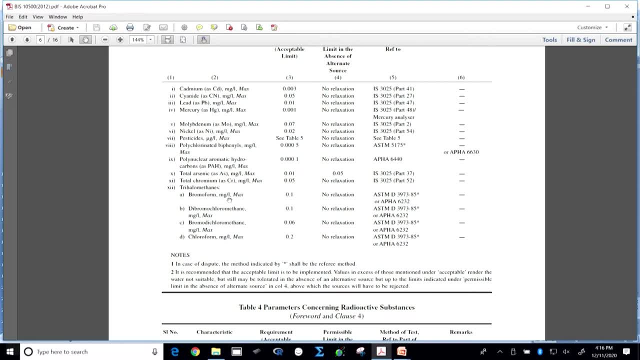 By-products which are given here In India. we have it at 0.1 milligram per litre for bromo foam, which is 100 nanogram per litre or 100 ppb. Here is total arsenic. As you see, it is pretty. 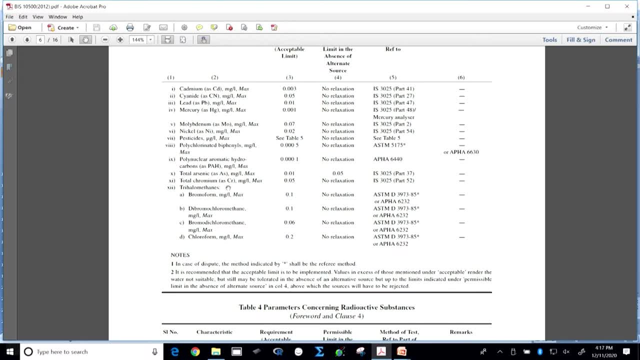 low 10 ppb. and same case with chromium- total chromium. Why total chromium or total arsenic? Because arsenic and chromium exist in different oxidation states. Here we are talking about total chromium and total arsenic, Typical way to analyse these heavy metals. 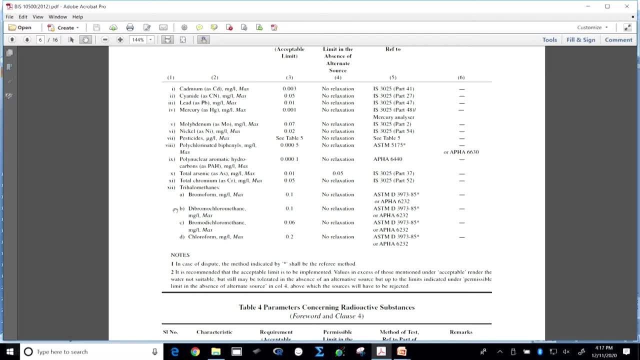 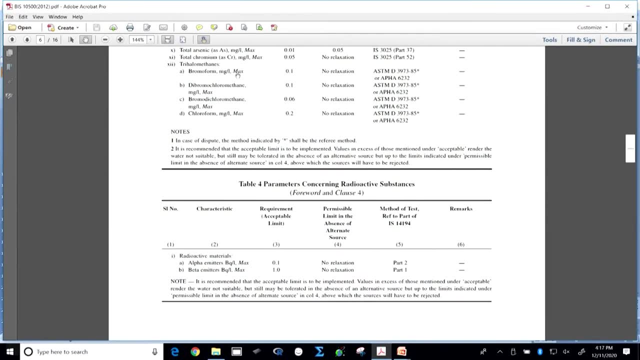 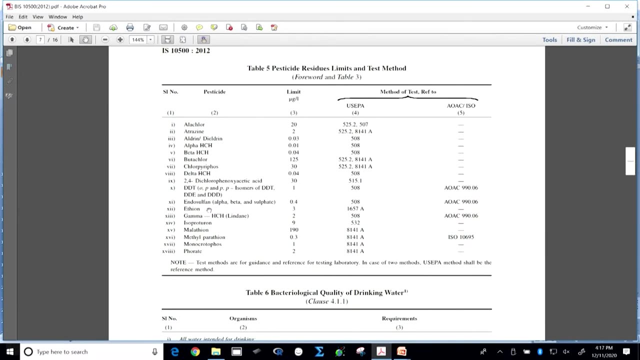 is by using AAS or ICP-OES or ICP-MS. Cheaper method is to use AAS- atomic absorption spectrometry. We have the trihalomethanes radioactive substances. Rarely will they come into the picture. I am not going into that. Pesticides typically based on Indian context or 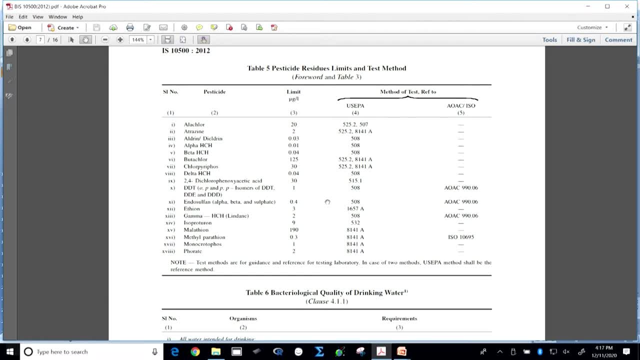 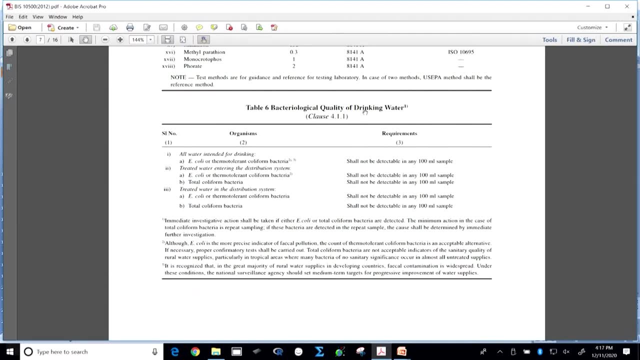 Indian, or information from or experiences from India. That is why we look at these particular compounds. Here we come to the bacterial quality. Note that we are talking about E coli, thermotolerant coliform bacteria, In general. we do the total coliform bacteria. Why are we going to look at total coliform? 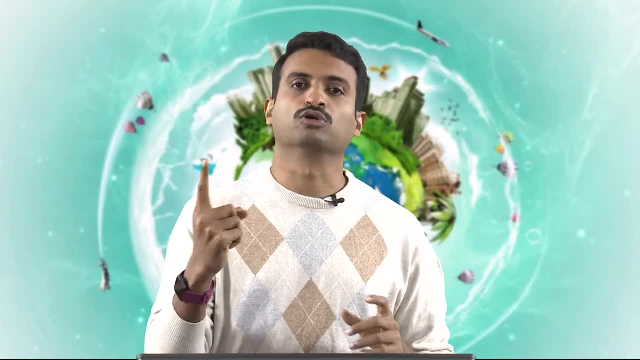 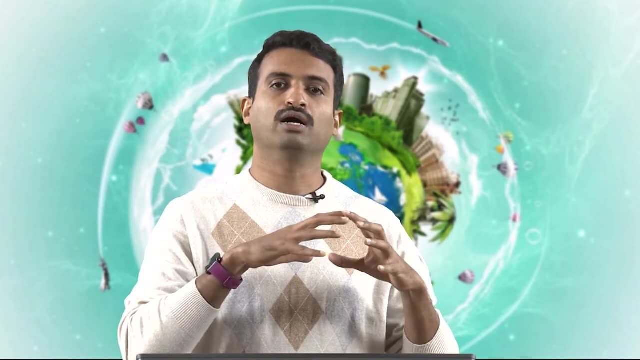 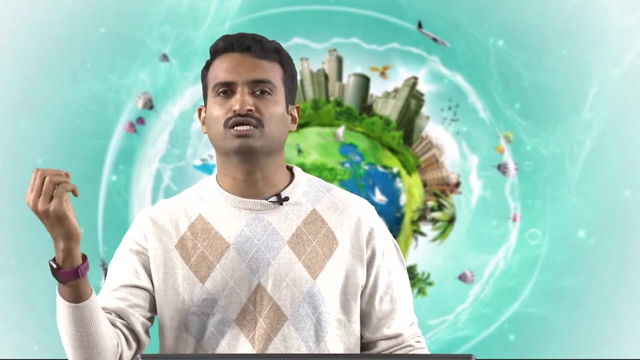 In this context, we need to mention that we looked at total coliform and faecal coliform, two relevant tests. Total coliform encompasses this faecal coliform. Fecal coliform we look for when looking at sewage treatment plant and water. from that Here we look at total coliform. 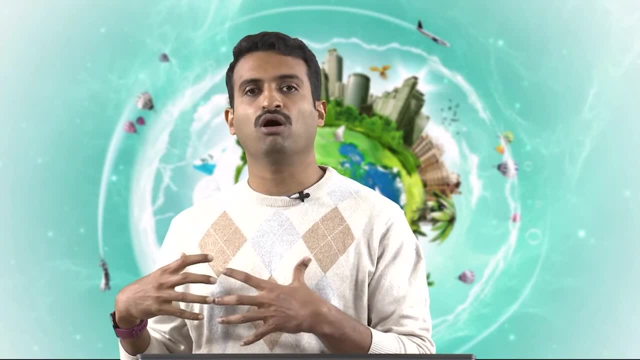 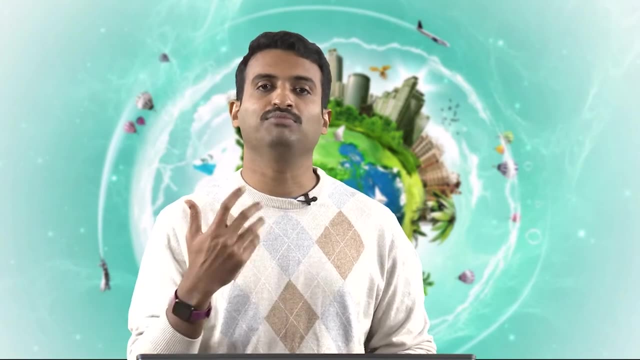 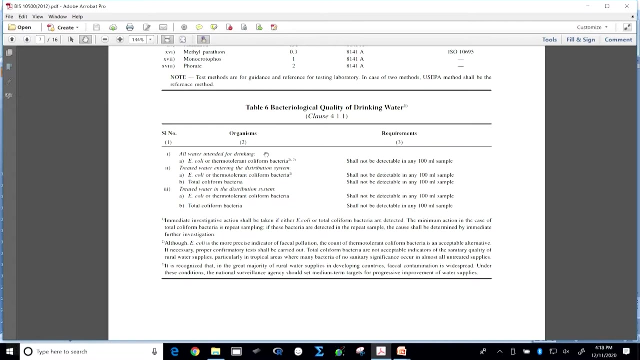 Total coliform. why is it? Because these are indicative of gut bacteria or faeces coming in contact with this water or contamination due to human faeces. What is the limit, As you can see, for all the kinds of uses: all water intended for drinking, treated water. 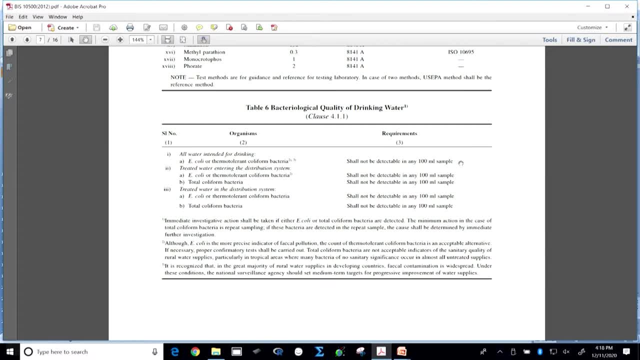 entering the distribution system: treated water in the distribution system. everywhere you see that it should be 0, not detectable in any 100 ml sample. Why 100 ml? Because it is based on the MPN test, But in any 100 ml sample it should not be present. That is the relevant aspect. 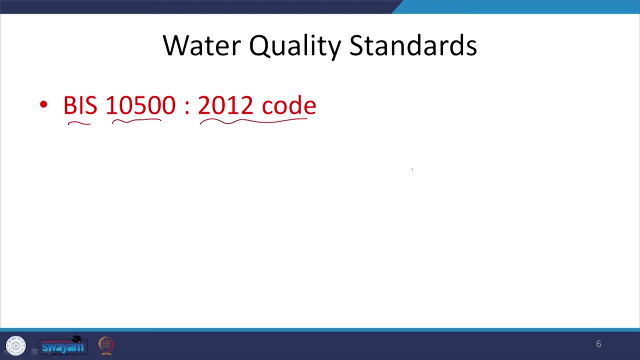 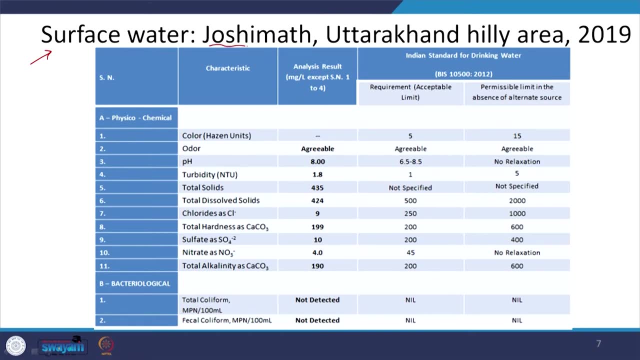 Let us move on or come back to where we were. Let us get this started. Sample water quality report, I think, from IIT, Roorkee of water from Joshi Bhat, I think, lower Himalayas in Uttarakhand hilly area recently. Let us look at what we have. 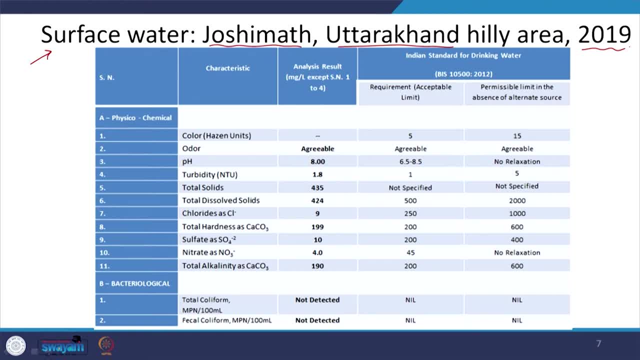 When we say water quality- typically at least, this is what we do or people in our lab do- What are we looking at Colour? we are typically not measuring that. unless it is visible, Then we do that units. There is a particular way to be able to do that with a spectrophotometer Order, just by using the 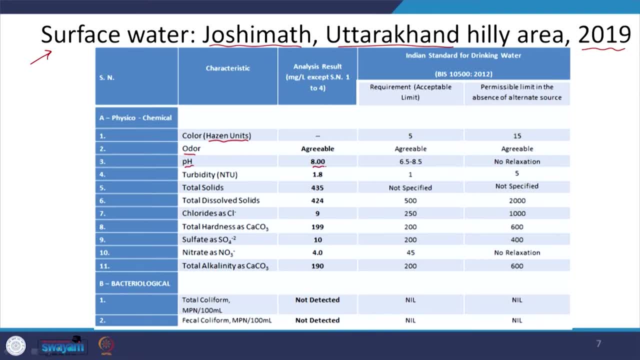 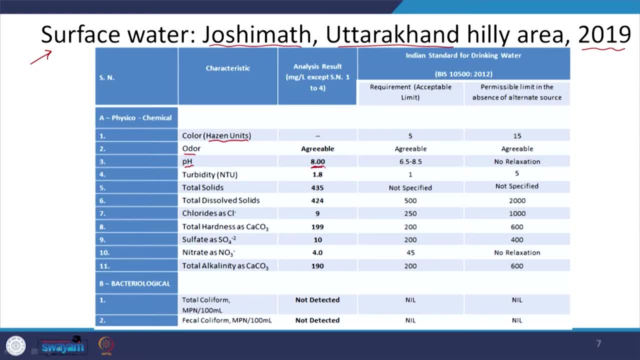 other deposits that can lead to decrease in concentration of H plus or increase in concentration of H plus and thus decrease in pH Turbidity. even there we see that it is 1.8,. acceptable limit is 1. And here 5, but please note that this is 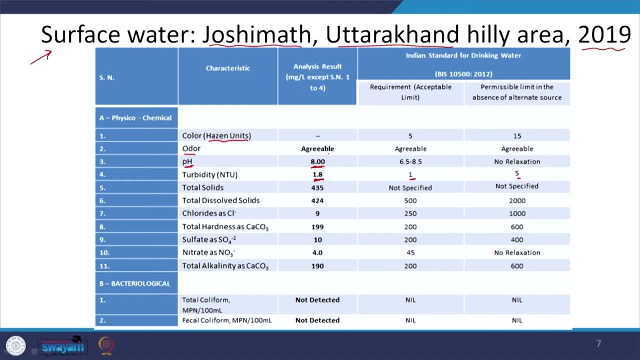 right from the stream, right without any treatment. So you know, along with the flow of that stream maybe some particles would have been kicked up and such, but you do see that there is still turbidity. In general we look at turbidity as an indirect correlator or variable that has correlation with 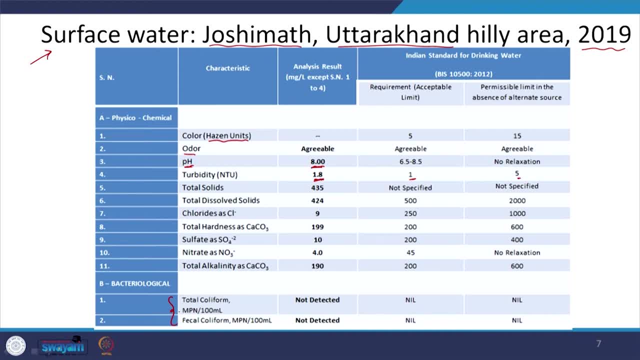 coliform or the pathogens. So again, we will come back to that later. Total solids: 435,. total dissolved: 424.. Keep in mind that if we look at these values and sum them up and play around, sometimes these values might be off. But again the issue is that when we are looking at this, 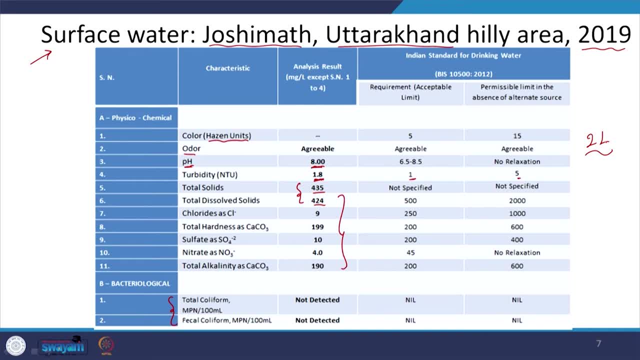 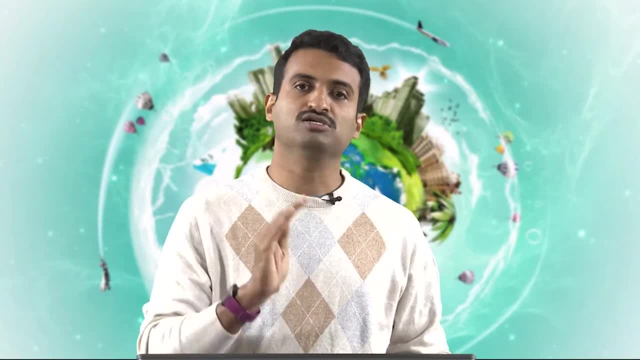 test. typically they take 2 litre water and then try to, you know, distil, not distil- filter and then put in the oven and such, But again, the accuracy is going to be pretty much affected, especially when we look at these concentrations which are so low. let us see. So that is one aspect. 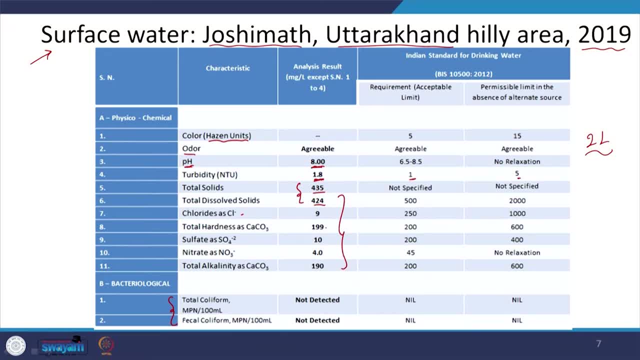 to consider. Chlorides obviously tend to be less and all other aspects are within the reasonable limits. let us say So. that is something to keep in mind. And, more importantly, what about the total and the fecal coliform? here We seem to be measuring both In general. total: 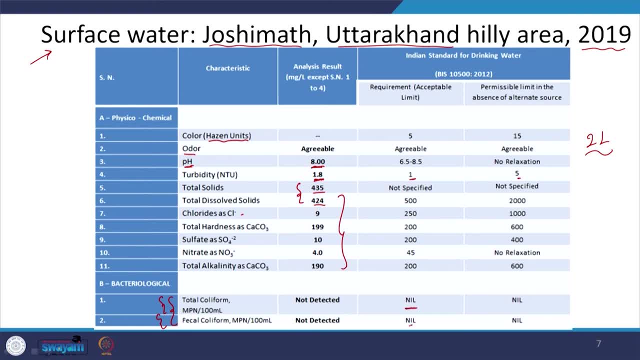 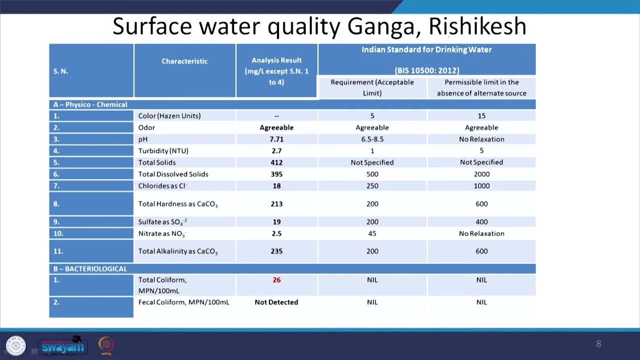 coliform is what you measure. Both came up to be nil, So this water is good for consumption without treatment too. So that is one aspect to keep in mind. Maybe, if there are sand particles or such, Yes 14, you can filter it with a cloth, but you can use this. But when it comes to Rishkesh water quality, 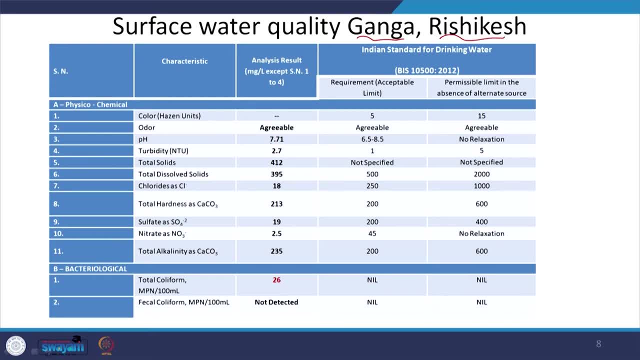 of Ganga at Rishkesh. what do we see here? pH is relatively less expected. turbidity has increased. it can be due to the suspended matter or due to other aspects which we will look at later. Total solids, dissolved solids, seem to be fine, all the other aspects to be more or less fine. 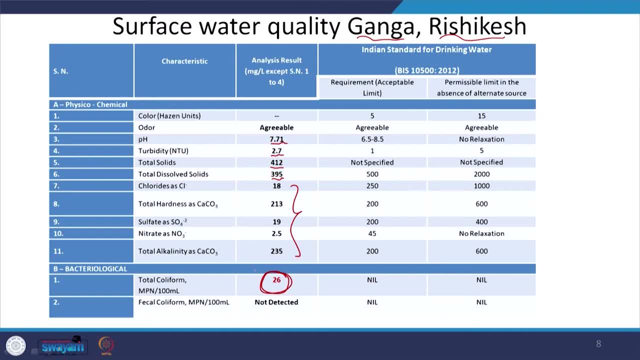 But, as you can see, the issue here is that total coliform 26,. even though fecal coliform have not been detected, you do see that total coliform is there. It is indicative of gut bacteria or contamination by human feces. If not human feces, more or less gut bacteria, if I may say so. 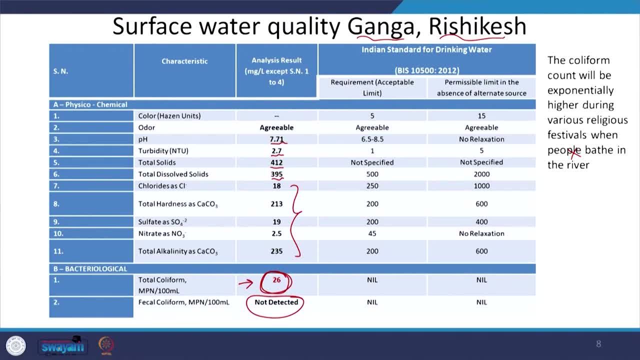 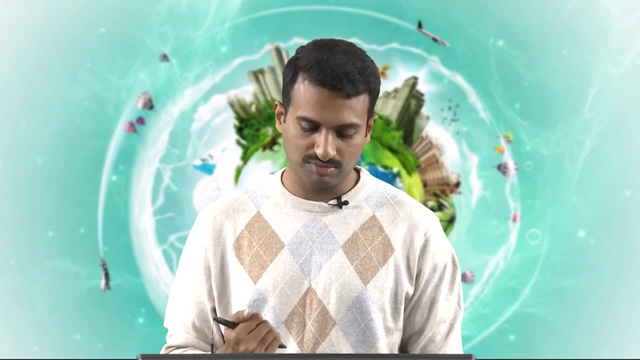 This water is not fit for drinking. And one other aspect is this: coliform, both maybe fecal and total- will be exponentially high when it comes to water quality. we have different religious festivals, when people have or come to bed and you have the melas, and that is when you are going to have it to be remarkably high. So you see the relevant. 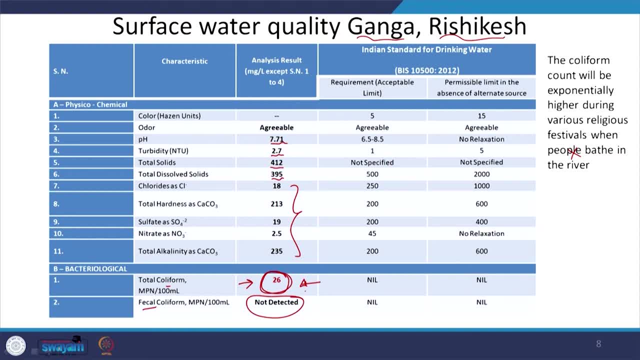 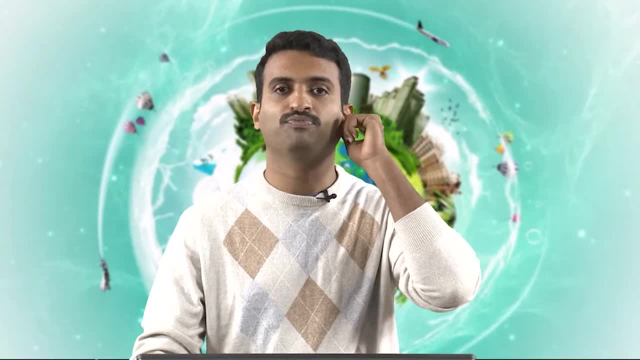 aspect, even though the water might look good, You see that we have, or we need to be concerned because there are considerable indicators that say that this water has pathogens, and that is one aspect to keep in mind. And in this context, you need to look at turbidity- Turbidity again. 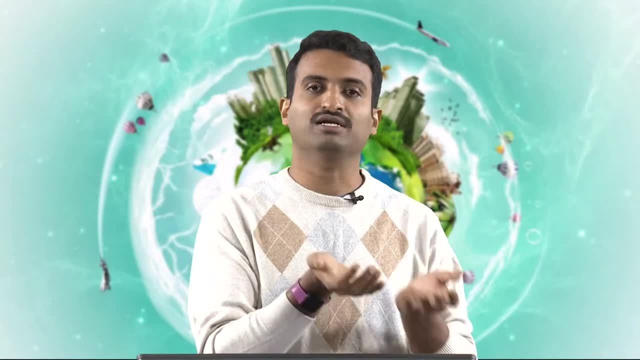 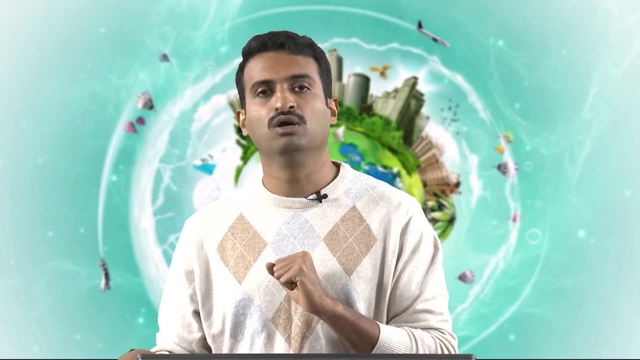 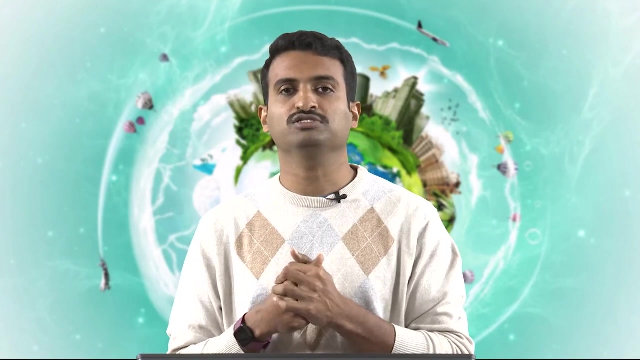 looks at how well the light is being scattered by the particles in that water And typically we look at a particular size of the particle- I think 50 or 5 micrometers or microns- And that particle size is more or less very much near the particle size of most pathogens. 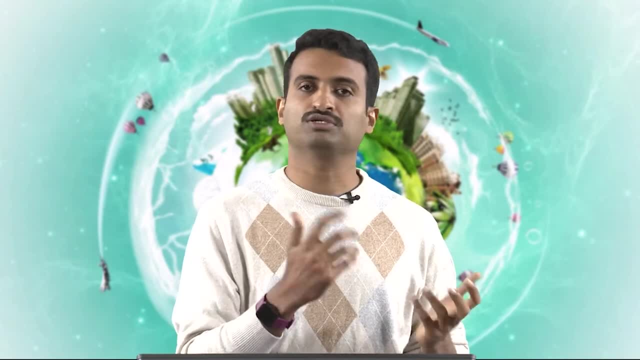 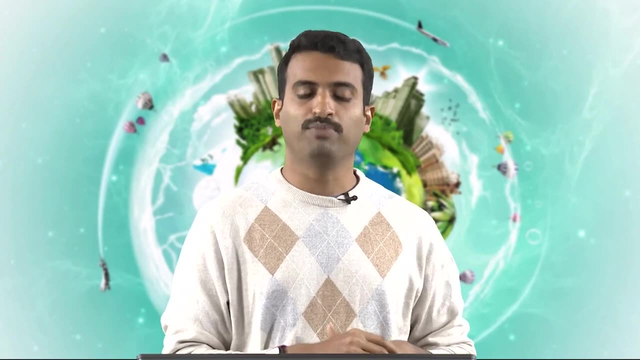 And that is why turbidity in drinking water, or at least in treated water or even in general water from the surface. you can use that as an indirect correlator for the pathogens. We will come back to that later, But I wanted to mention thatanno. 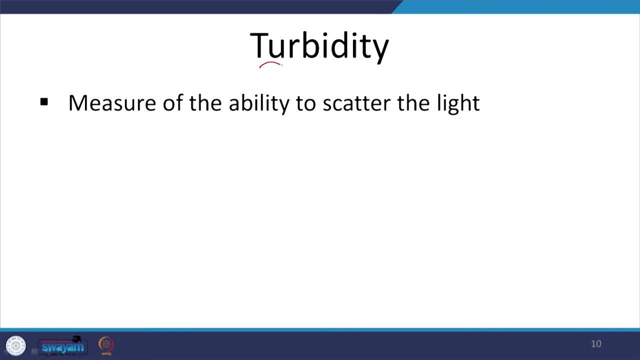 So what are some of the other important parameters? So turbidity, what will it give me an idea about? it will give me an idea about the ability of the water to scatter the light. Why is this concern? So I have this small particles in water, So it comes through. 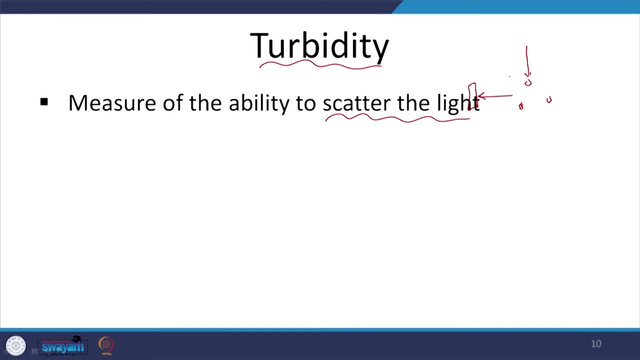 is particular test. Well, How this detector here, so at that 90 degree angle, how much light is being? what do we say scattered? So some of particles from the water that have been scattered. so some, that is what it will measure. So what are the causes? It can be inert, like clay, silt and some. 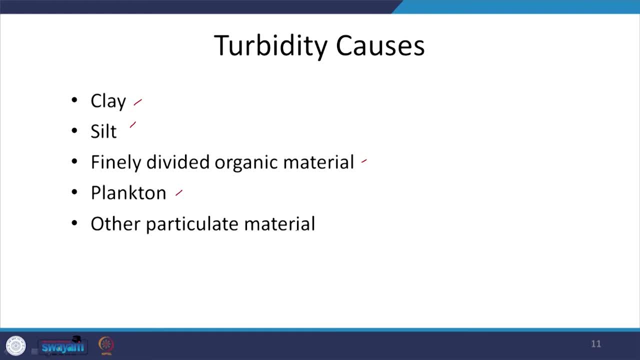 organic matter which is not inert. It can be plankton, It can certainly be pathogens, Some pathogens and other particulate matter. So on these organic or especially on particulate matter or on clay, you can have pathogens thriving. So that is one other aspect to 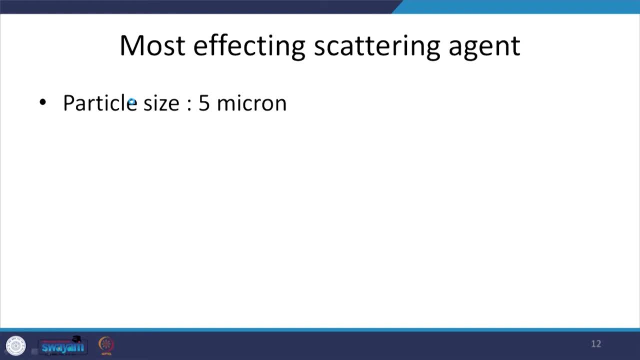 be aware of, So most effective scattering agent. the size is 5 microns, as I mentioned earlier, and this size closely matches with the size of your pathogens Unit and measurements. we have a turbidity meter which is pretty easy to use and the reference is: 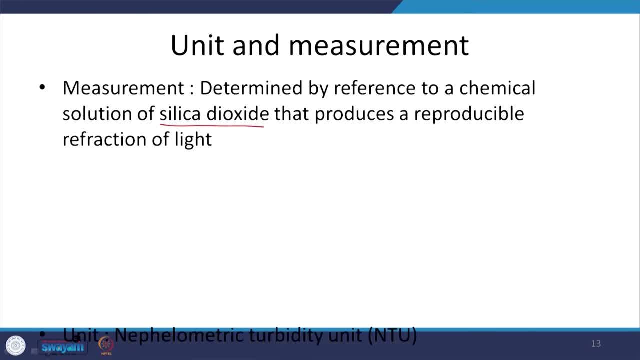 the solution of silica dioxide And we use turbidity meter. the units are nephelometric turbidity units or NTU. That is what you see, and turbidity in excess of 5 are easily detectable in a glass of water and are objectionable for other reasons, such as aesthetic reasons. 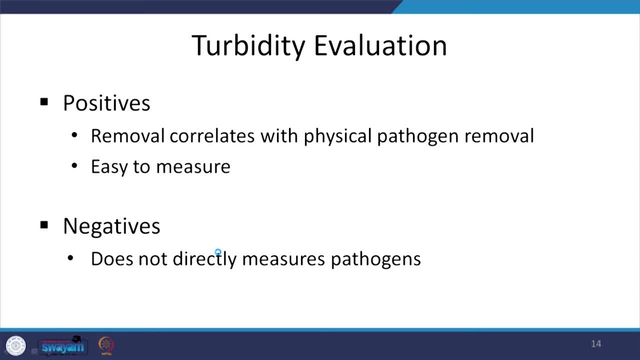 So that is something to keep in mind. Let us move on. Why do I need to look at turbidity? As I mentioned, it correlates pretty well with physical pathogen removal. let us say turbidity 10 and pathogen of 100 or so, Turbidity 2. 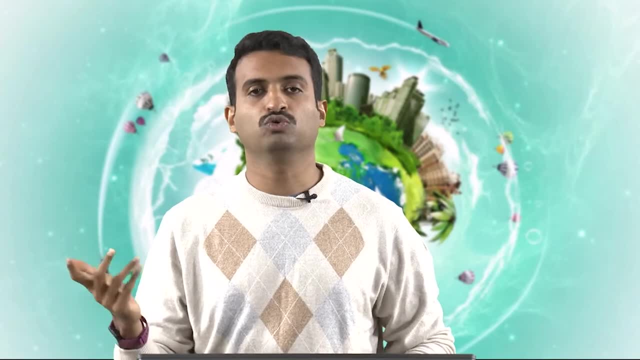 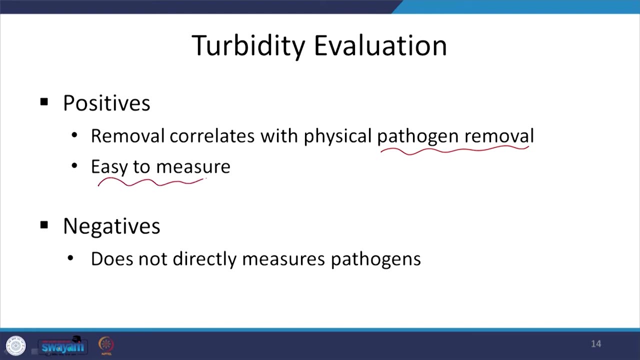 or 1 and pathogen of almost 0 or 2 or 3.. So that is one aspect. it correlates, So correlates pretty correlates pretty well with physical pathogen removal. And more importantly, as I mentioned, you know, you even have these handheld portable. 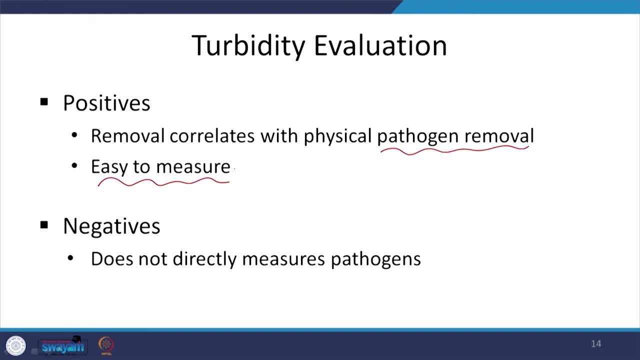 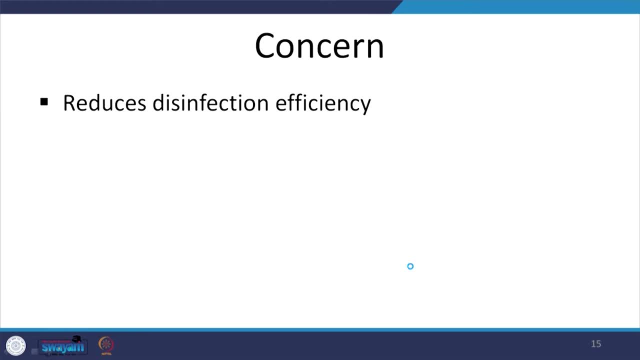 turbidity meters. it is pretty easy and cheap to measure Negatives. obviously it is only an indicator which correlates. it does not directly measure the pathogens. right, something to keep in mind. So another aspect is, as we looked at, we can have UV and if we have, 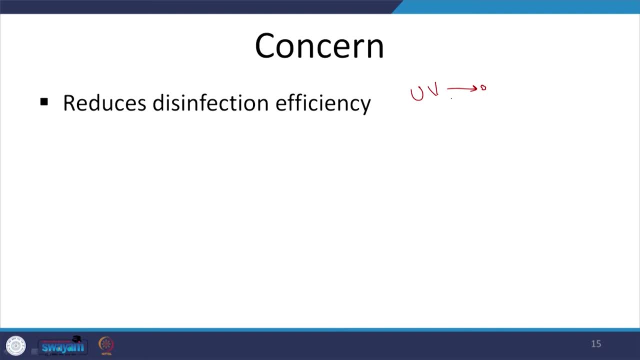 UV and turbidity. why UV? I want to disinfect the water, you know, and my relevant pathogen is here. right, my pathogen is here. So the UV will be absorbed by the relevant particles, leading to turbidity, or the pathogens will be shielded from UV. 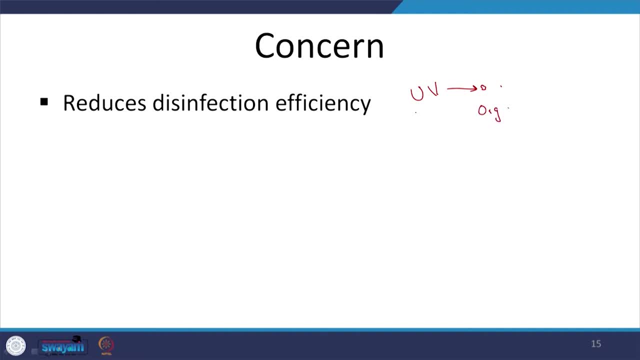 Same case if you have organic content, organic matter, and I add other oxidizing agents such as, let us say, chlorine or HOCl or ozone, right, These organic matter which will be taken up by or can be measured indirectly by, turbidity, suspended organic matter anyway. 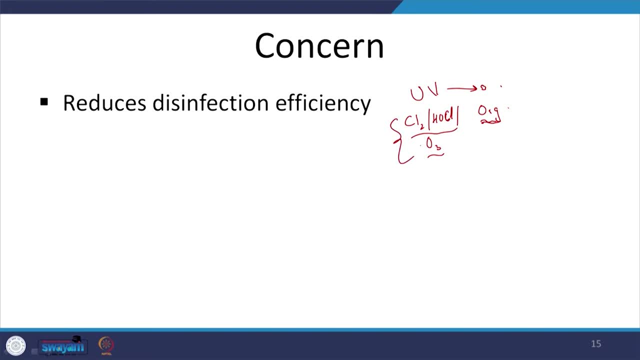 will consume the oxidizing agent, thereby limiting the disinfection efficiency. something to keep in mind. So, pathogens: typically we look at total coliform. we do not look at faecal coliform. faecal coliform is a subgroup within total coliform, So it also includes what do we see? microorganisms. 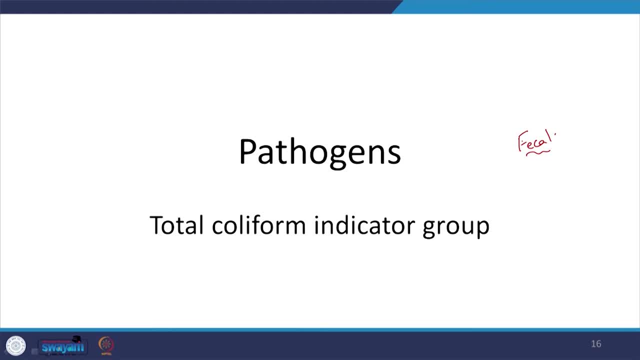 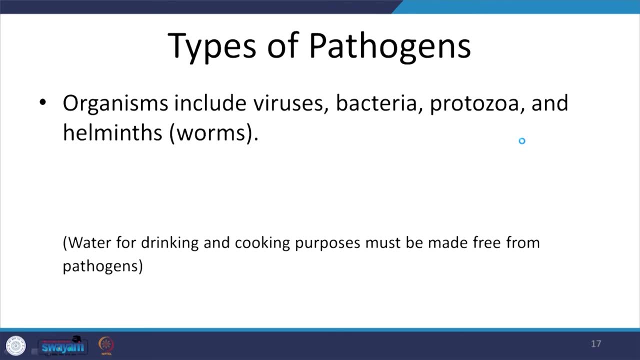 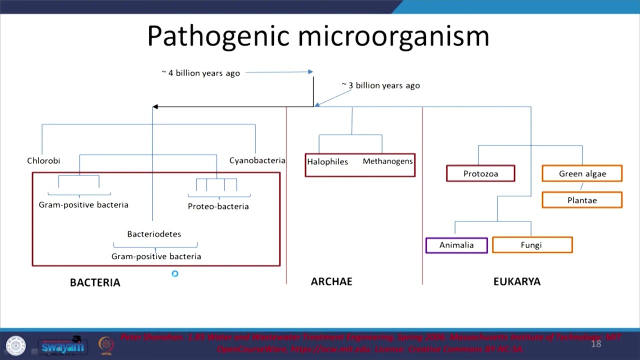 from roots of plants and such, if I am not wrong, And also from the guts of warm blooded animals. so which includes human beings? too right, The organisms include viruses, bacteria, protozoa and helminths. Yes, and in general we look. 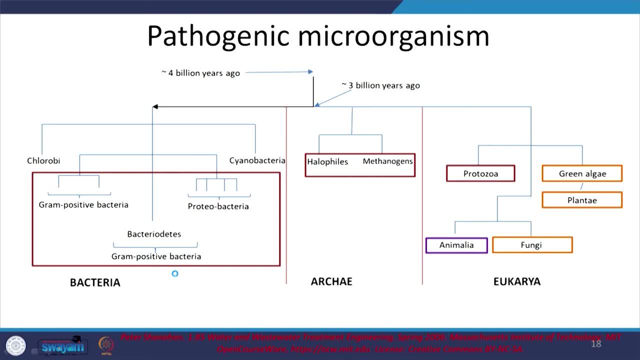 at. okay, we looked at this figure earlier And in general, we are concerned with these bacteria, some of which can be pathogens- the one silated and protozoa- I think we looked at this- cryptosporidium sporidium and giardia. 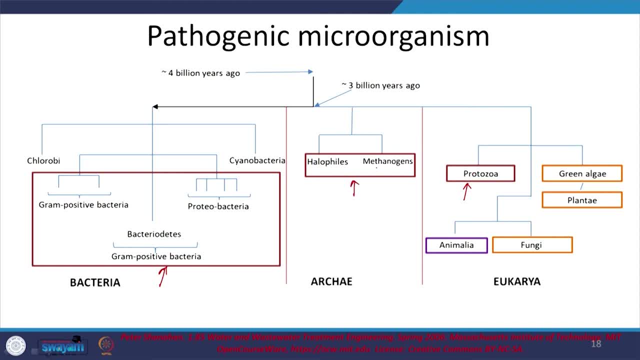 And in the context of environmental engineering, especially in the context of anaerobic treatment. we look at methanogens, but typically RKA. they are not a concern with respect to drinking water quality, with respect to health concerns, but we are concerned about these bacteria and some of these eukaryotes. That is something to keep in mind. viruses, too, viruses which 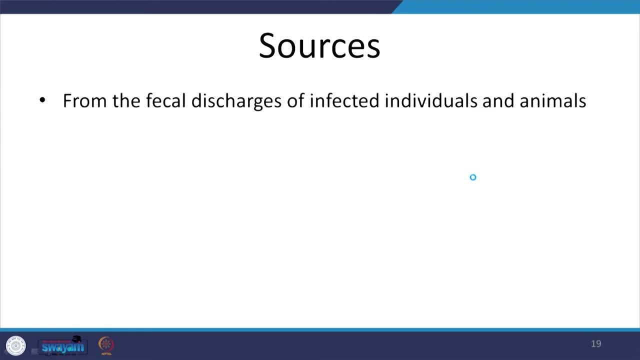 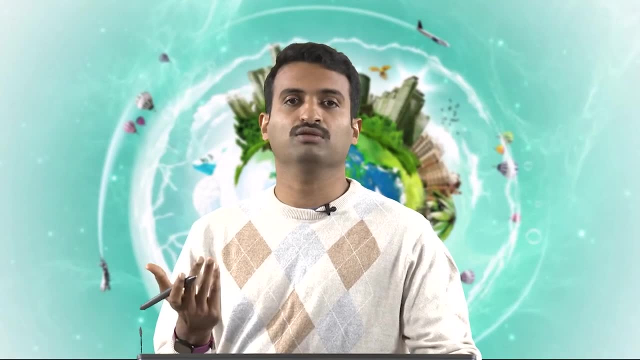 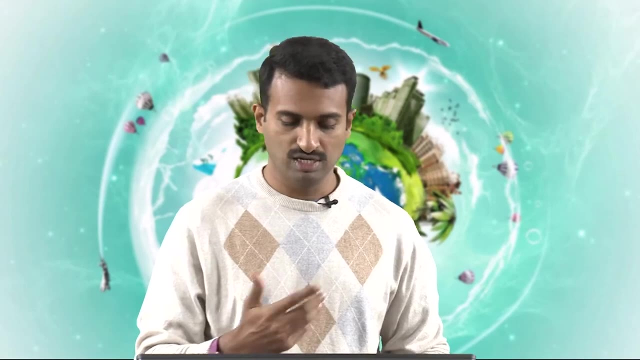 are not mentioned out here. let us move on. What are the different sources by which you can have contamination of the water by pathogens? Typically, it is the fecal matter of an infected individual coming and mixing with the drinking water of another human being. That is what we have out here and this test in estimates. 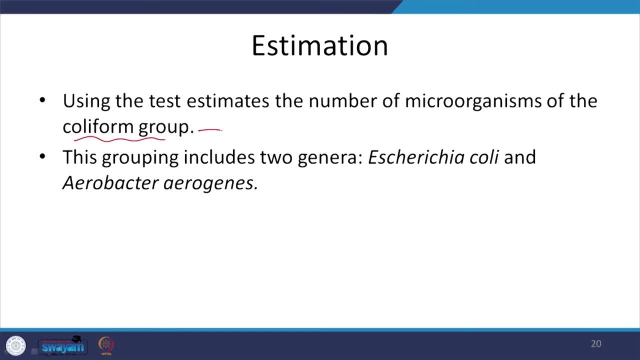 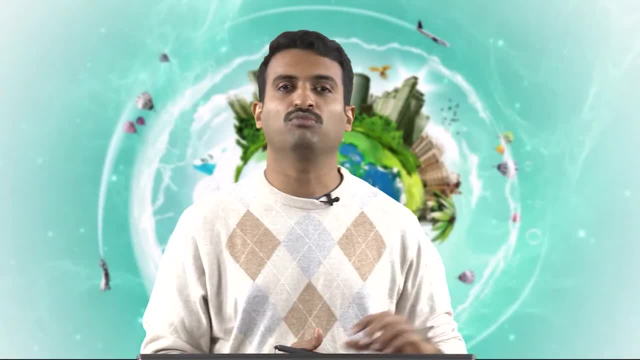 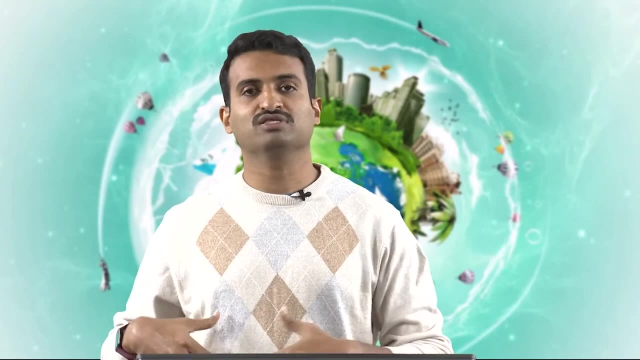 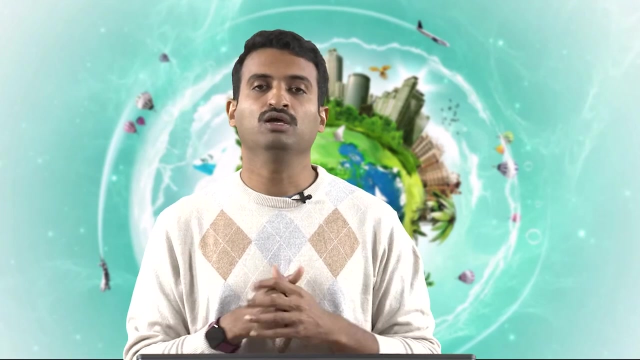 the number of microorganisms of the coliform group which are an indirect indicator or indicator of pathogens. Why do we look at this coliform or this indicator organism? Why did we, or people, choose coliform? because it correlates very well with the pathogens that we release or from which are- from our gut or from our feces. it correlates very well. 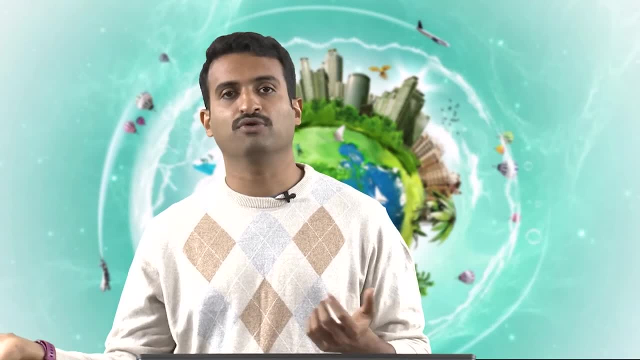 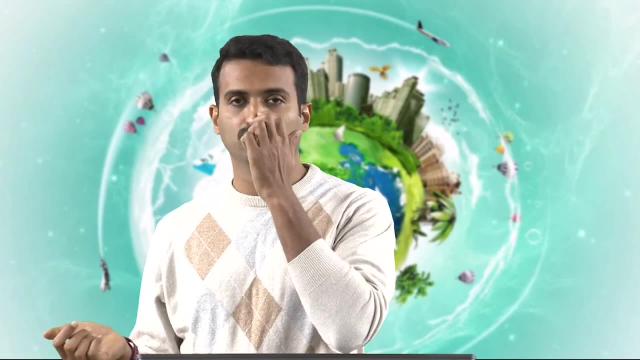 and, equally importantly, it thrives well outside our human body. It is not as if it thrives for longer time only in the body. then if I cannot measure it outside, in the environment or water, it is of no use. It can thrive well there and it is easy to measure too. 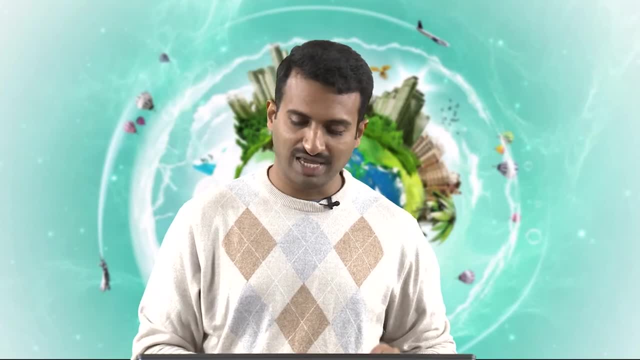 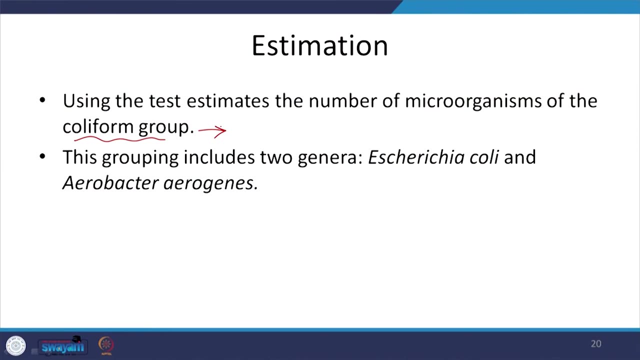 Relatively easy to measure, Very easy, if not very easy. These are some of the aspects why we choose to measure or look at the coliform group to understand or to try to see the presence of pathogens, and thus looks at E coli, for which we also find a mention, of which we also find a mention in the standard, and aerobacter aeroginous. 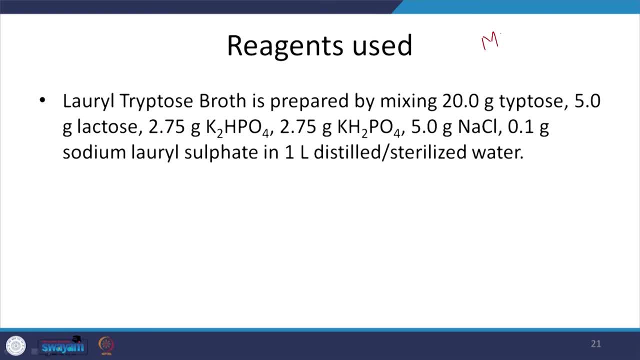 And reagents used in this test. typically we look at. there are other tests, MPN, most probable number- that is what we typically look at And we have specific type of growth that is conducive for these. coliforms is prepared And we have the tiptoes- lactose and different phosphates and nutrients and you prepare that. 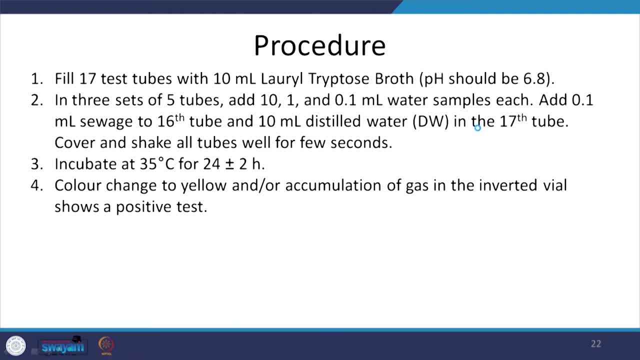 again, you do not need to mark this up And you are going to fill 17 tubes, but in general it is 5 times 315 right plus 2, why 2.. We have 16 tubes where we add sewage 2. 2.. 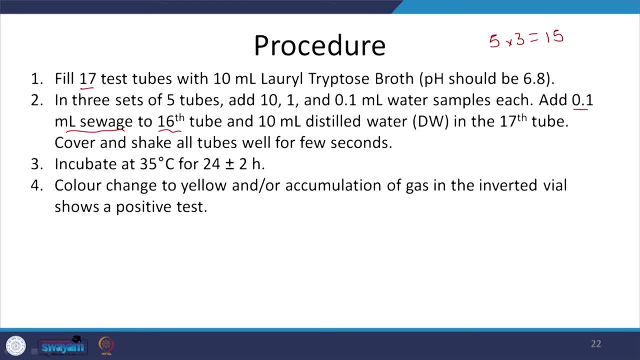 whether the test is coming out to be right or not, so that it is a reference. This is not standard or required, but that is what we do in our lab here. And 10 ml of distilled water to see that there is no false negative or false positive. Cover and shake all tubes. 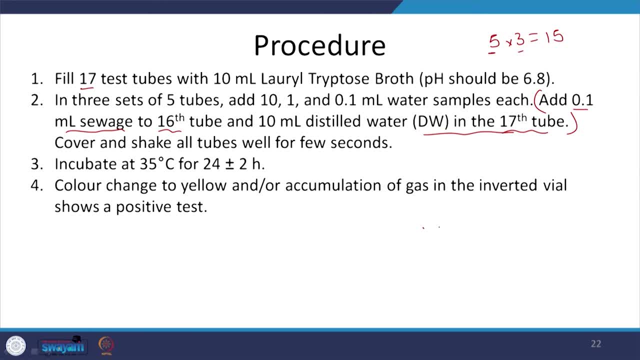 well for a second In these sets: 1,, 2,, 3,, 4, 5,. 1,, 2,, 3, 4, 5,, 1,, 2,, 3,, 4, 5.. 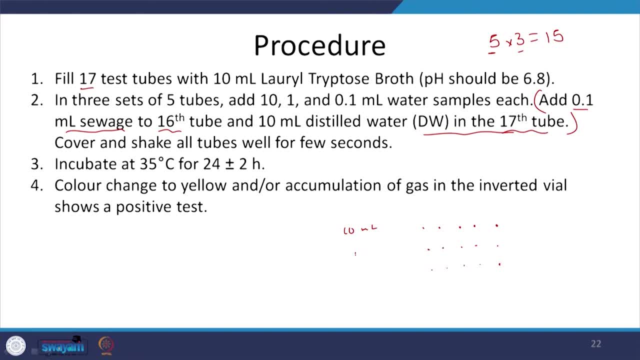 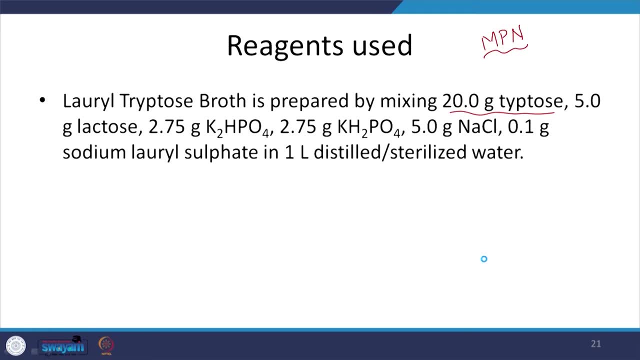 In the first one, I add 10 ml of the waste water. The second one, I add 1 ml of the waste water. In the last set, I add 0.1 ml of waste water and also I add this broth that we prepare. 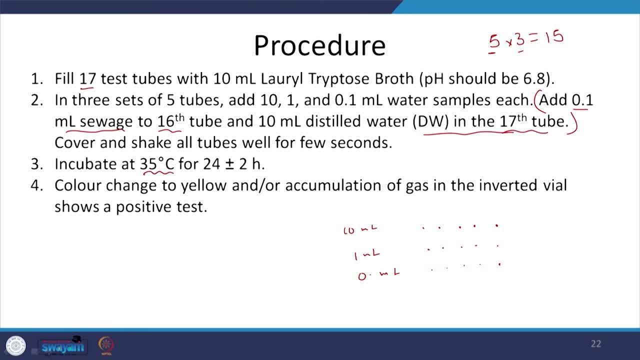 And then we incubate it at a particular temperature that is conducive for growth for a sufficient period, which is 24 hours. When the colour changes to yellow due to the acid being produced or accumulation of gas in the inverted vial, it means that there is a positive. 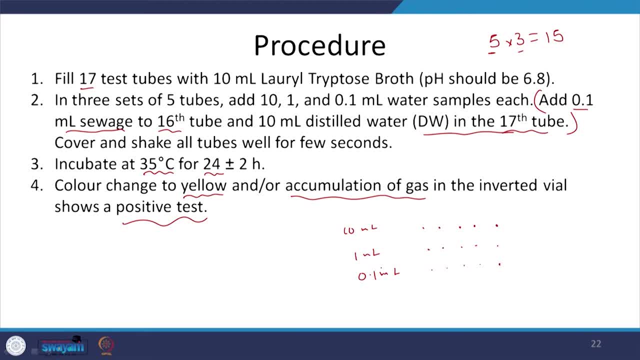 test You can have. sometimes, depending on the kind of sample, you can have a positive result here but negative results in all the 0.1 samples here. Why? Because it is not that you have uniform distribution of the pathogen in the relevant or the coliform in the relevant sample. 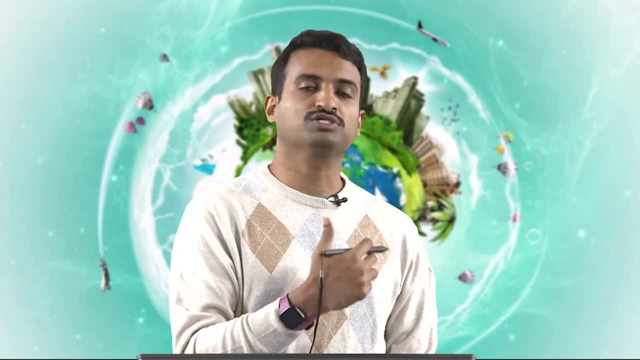 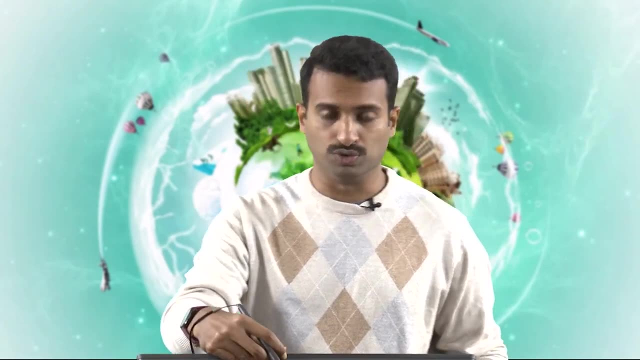 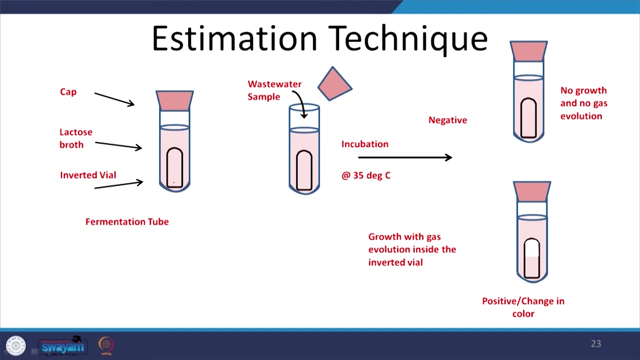 Here there is, I would not say, guessing work. statistics is involved, but you have tables that will give you an idea about how to get this number. We will look at that soon. Let us move on. estimate pretty simple: Lactose broth, inverted vial to capture the fermentation products, the gas. 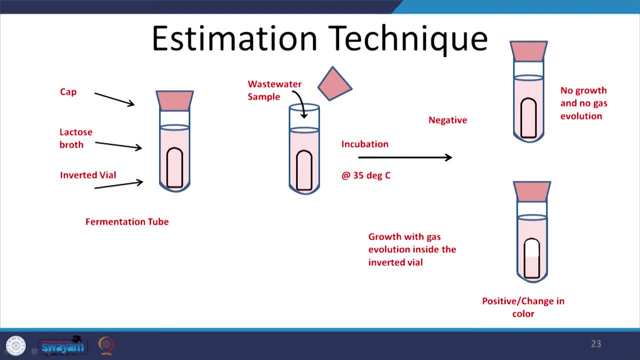 and fermentation tube by gas And waste water is put in 10 ml, 1 ml or 0.1 incubated. If it is negative, this is what it looks like. If it is not negative, you have gas and also you will have some. 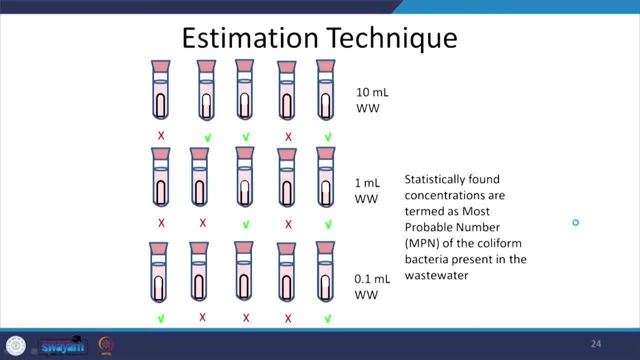 colour change here depending on the type, kind of test. You can have positives here positives and positives here, 10 ml, 0.1 and such. Based on that, we are going to look at it In general. what does it mean? Let me also. 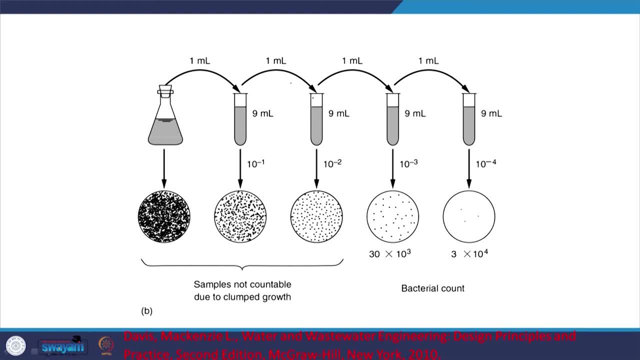 look at it: Waste water. we are diluting it by 10 times each, Each time, each step. we are diluting it 10 times The microbial count, or the microbes. also, it is supposed to decrease. That is what we. 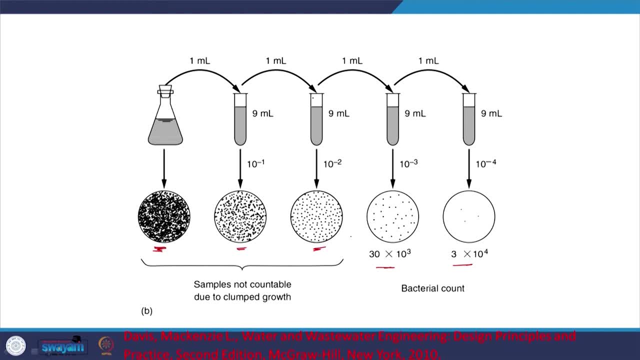 have Here. there are too many to count, too many, too many to count, Though we are not counting. some people can do this. You can count the. you can also come up with the bacterial count, But that is not usually done, but can be done Usually. what do we do? This is what 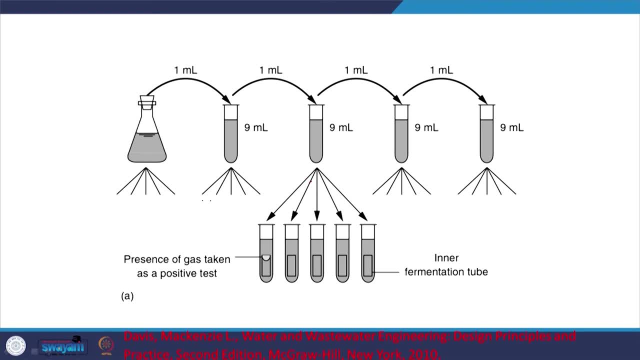 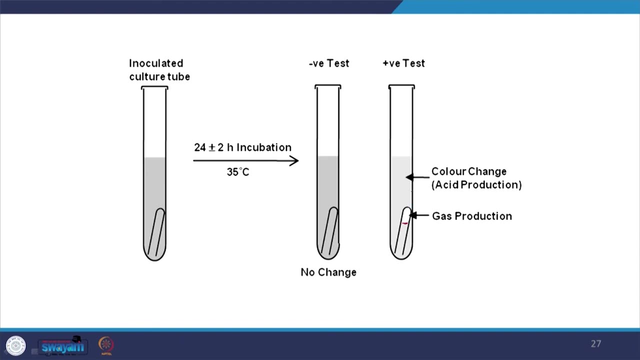 we do. We try to situate that. We put that dilution into these tubes for our MPN test. One set is out here. Different ways you can count, but this is what we do in general And where is the data? As we mentioned, if there is gas production and colour change due to acid, 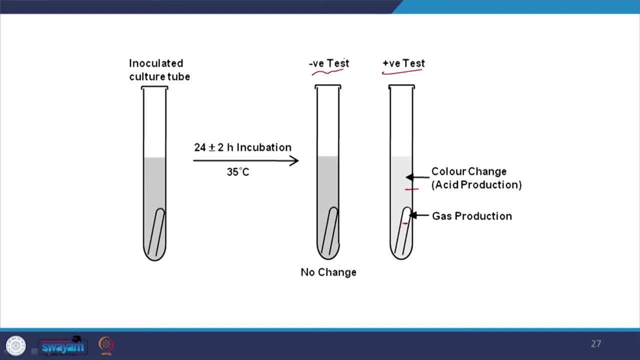 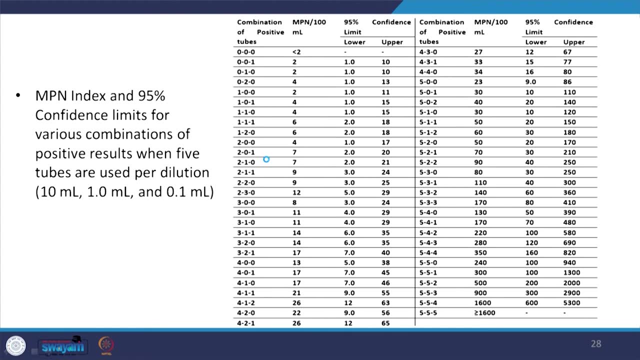 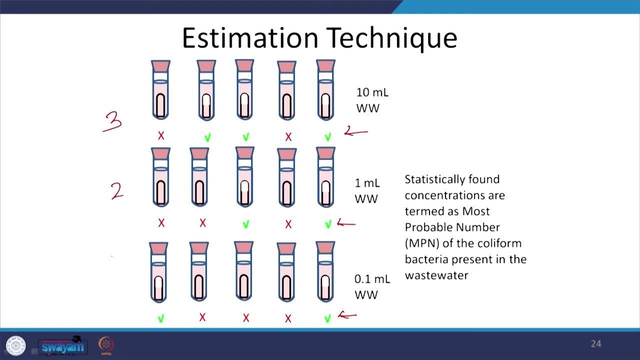 production: positive test. If there is no change: negative test. We are going to incubate for some time at the temperature. How do I get this? How do I get the MPM Here? it seems like it is 3,, 2 and 2 out of 5.. How do 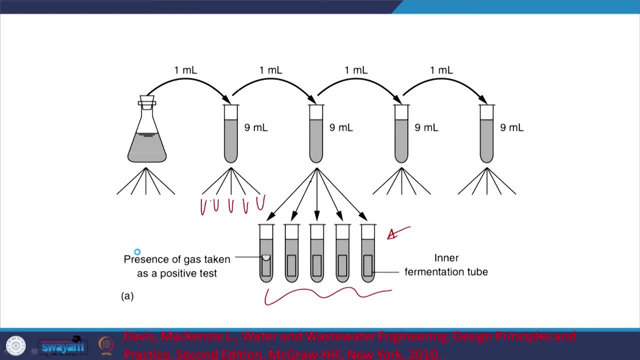 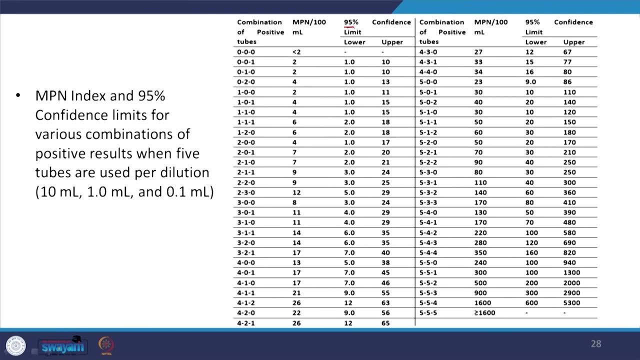 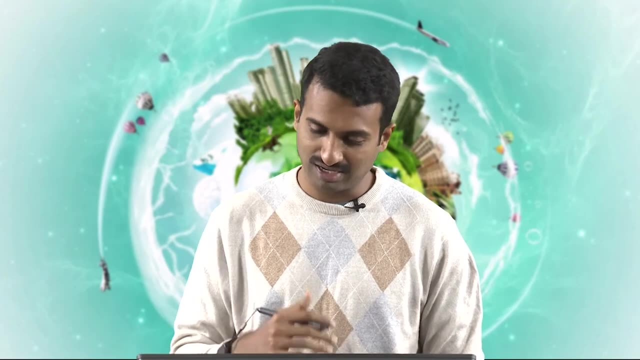 I get it Here. we are going to, I think, use the tables based on the Poisson distribution Here for a 95 percent confidence interval. Here we are not saying, with a 100 percent, what do we say? issue right, but it is at 95% guarantee, let us see all right, 95% confidence, I guess. 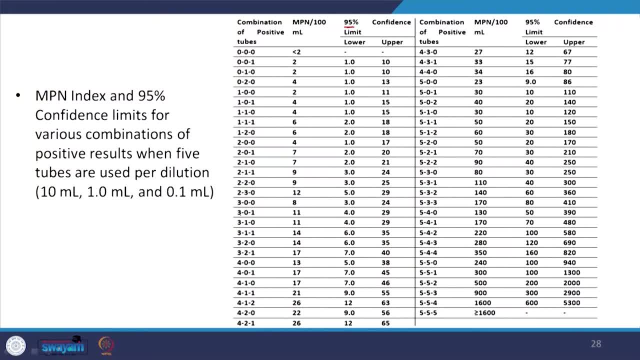 So we were looking at, I think, 322, right, so where is 322? okay, I cannot find 322 here. So anyway, let us assume that it is 321, okay, 321, yes, So MPN is 17, let us see right. per 100 ml. that is what we have: 95%. lower limit is 7 and upper limit can be 40. So, but typical one is 7, but lower limit is 7, 17, pardon me, lower limit is 7 and upper limit is 40. let us see: 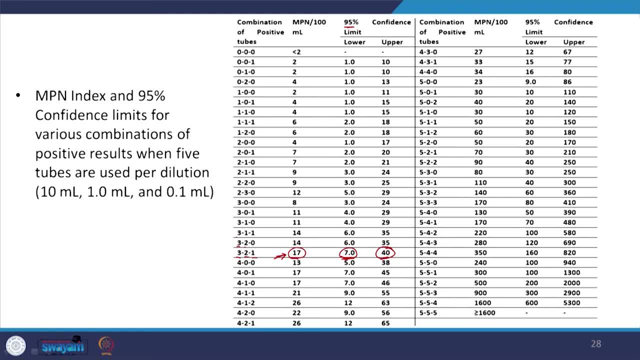 So, based on different- what do we say? combinations of positives, you will come up with this most probable number from this particular data. let us see right. So obviously, if it is all 555, you cannot just say it is 1600.. This you will see. let. 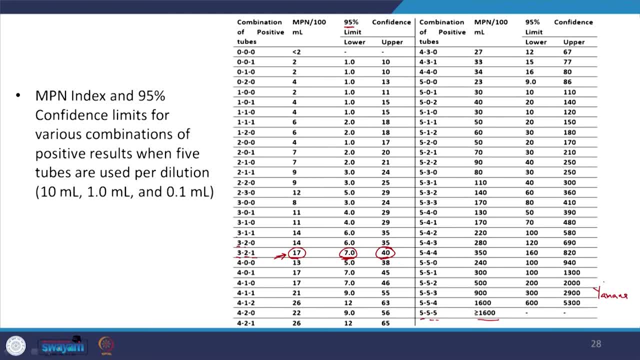 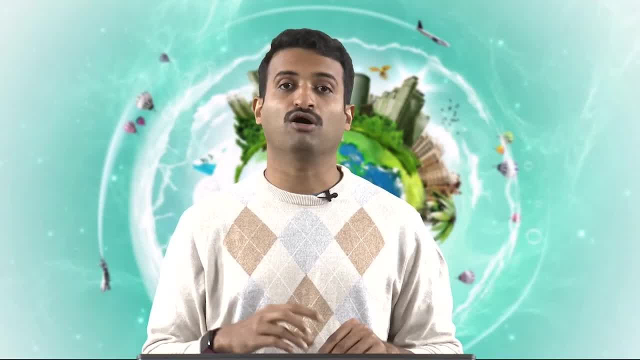 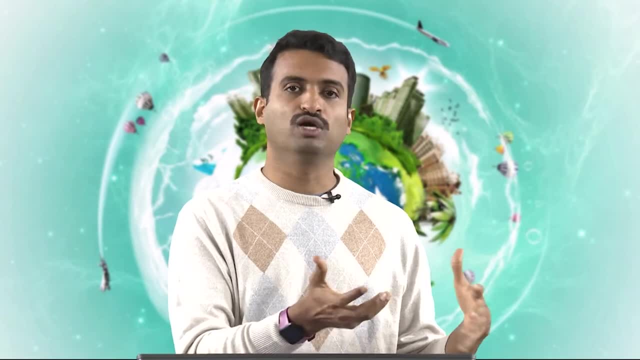 us say in Yamuna, I think, where MPN will say that it is in lakhs and lakhs, I think, if not millions. So that is because considerable untreated or partially treated sewage from areas surrounding Delhi which are not covered by Delhi sewerage network will come into Yamuna, downstream of Yamuna. So if you take a sample, 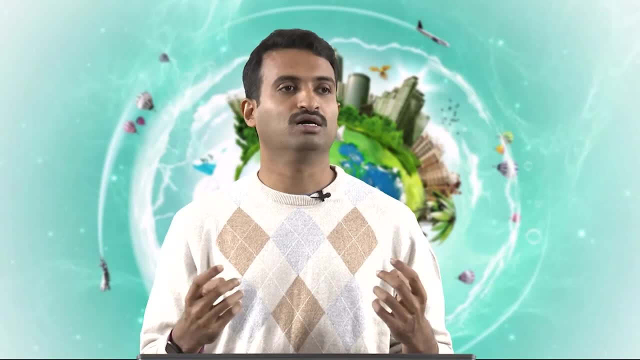 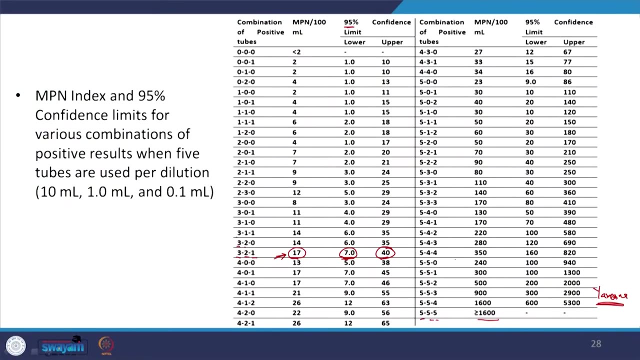 downstream of Yamuna, you will see that it is remarkably teeming with different kinds of pathogens and microorganisms. In that case, you will have to dilute that water a lot before you conduct this test. If it is all 555, what do you need to do? you need to dilute it so that you come. 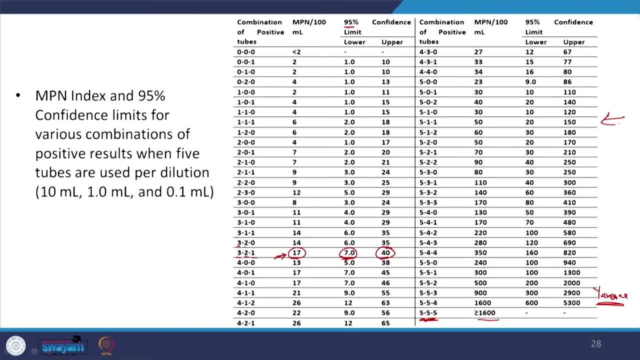 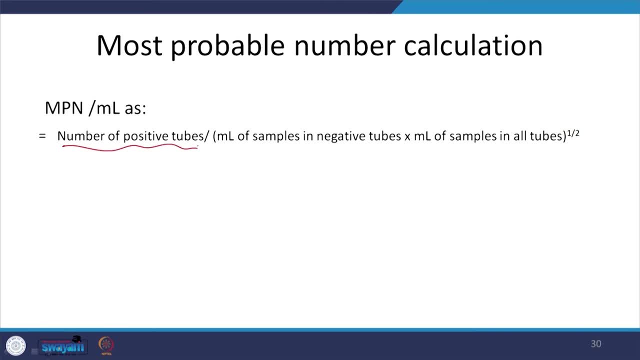 to a more measurable range. So estimation technique- we already covered that, if not another way- is number of positive tubes by the ml of volume of the sample in the negative tube, volume of samples in all tubes, square root. So this is another way to get the MPN number. So as we 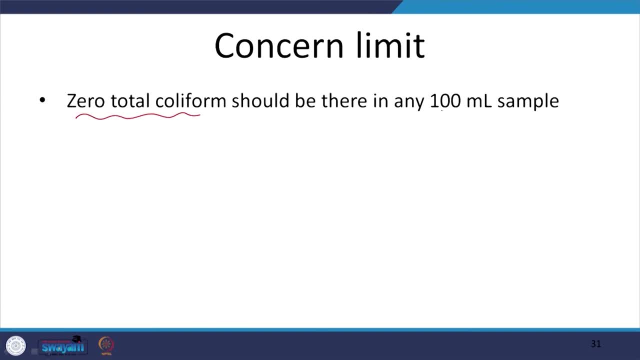 mentioned. what is the limit I need to be concerned about? it has to be 0 in any 100 ml sample. right 100 ml sample. So disinfection byproducts. okay, let me try to get this done, because we already looked at this earlier. So why do I need to be concerned about it? we already discussed this in the context of 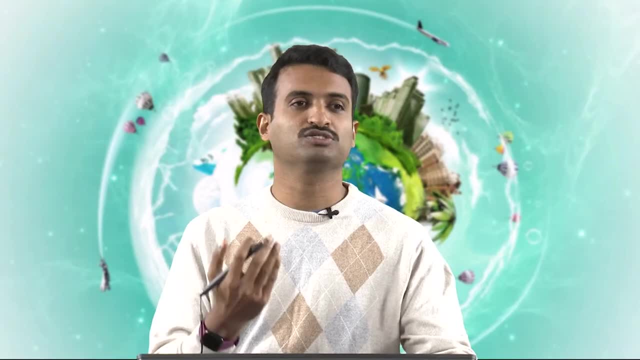 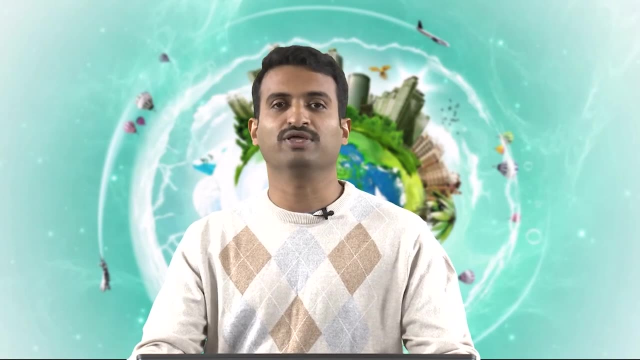 waste water I specifically mentioned. let us not chlorinate what we say waste water that is being discharged. but people do that here due to dubious reasons, when they cannot degrade the waste water well enough. But what do you need to be concerned about? it has to be 0 in any 100 ml sample right 100. 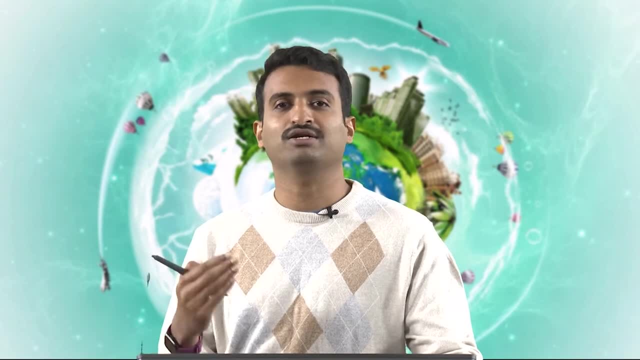 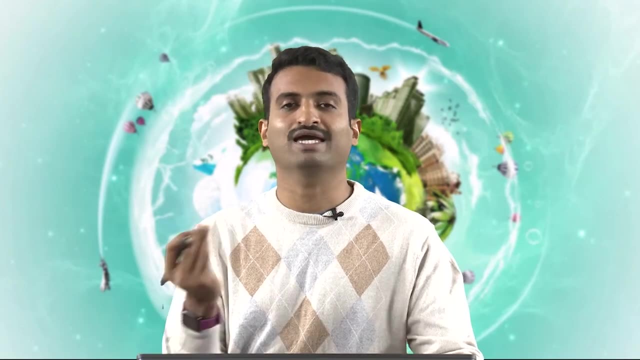 ml sample. So what do you need to be concerned about? it has to be 0 in any 100 ml sample. So what to show the relevant regulatory agency that they can treat the water? what do they do? they chlorinate it. when they chlorinate it, obviously you know the chlorine, which is a oxidizing agent, can oxidize. 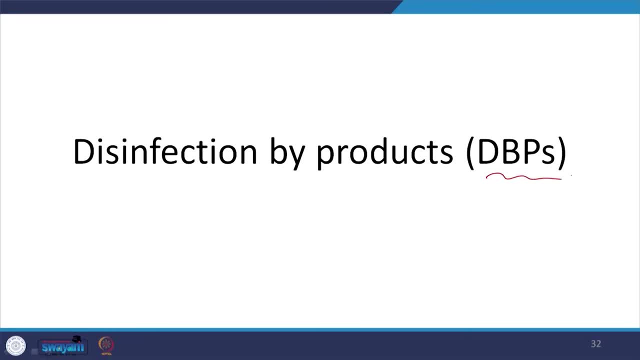 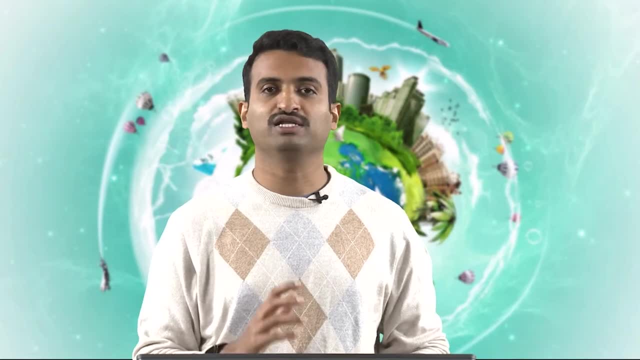 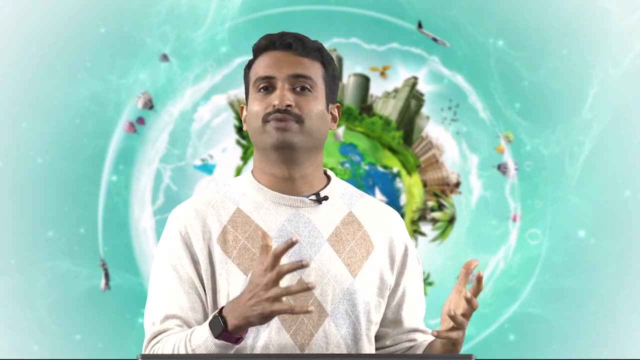 some of the organics, But you have very toxic or considerably toxic DBPs that are released into the aquatic stream. let us see For waste water. there are no standards for DBPs, but that is obviously what do we say? remarkably foolish thing to do from the environmental point of view. But 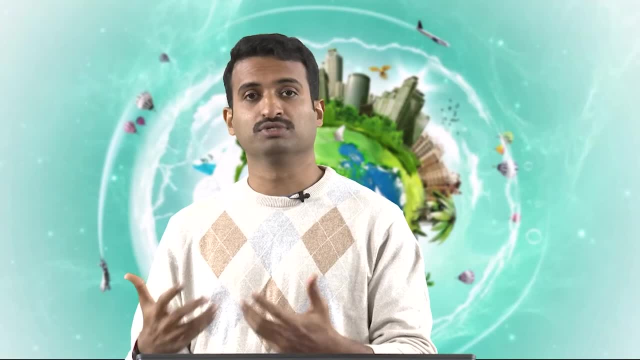 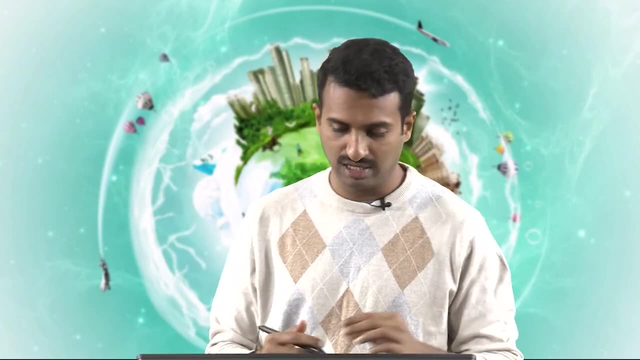 obviously people do not care a lot, but with drinking water it is toxic to me. So, as we saw in that bureau of Indian standards, we had the relevant limit specified for one class of it. So we already looked at this. how do we, how are these form disinfection byproducts? So byproducts? 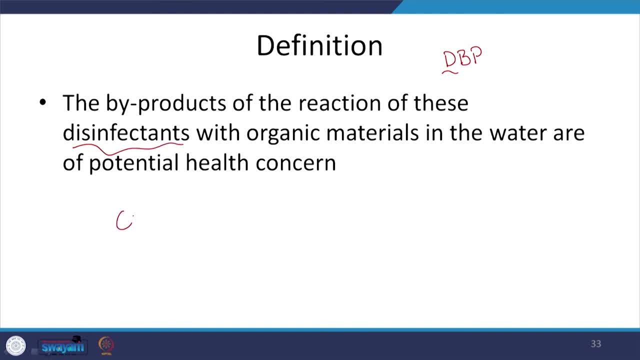 of disinfection when I am adding a disinfectant, typically Cl2, HOCl or such. when they react with organic materials. we have this. we already covered this in detail when we looked at the relevant DBP formation. So what do we say? remarkably foolish thing to do from the environmental point of view. 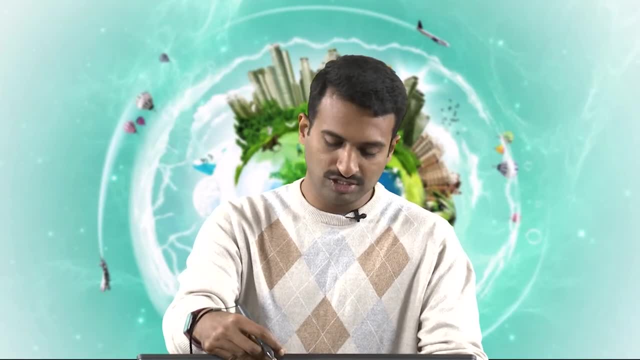 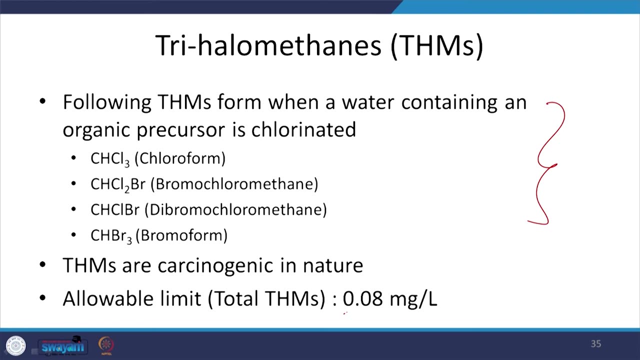 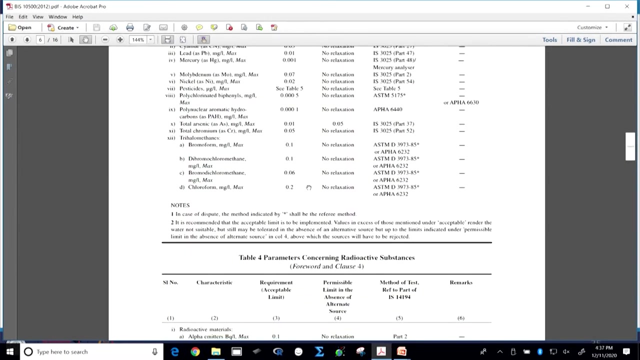 In the context of waste water or disinfection of waste water. So types of DBPs- in India at least, trihalomethanes are, what do we say? regulated. So I think this is not from Indian context. let me just check right away. right, where do we have that? okay, So obviously we have much higher. 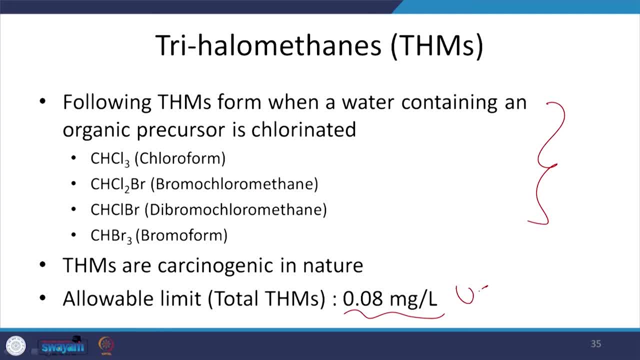 standards out here. So this is, I think, from US EPA. my TA might have forgotten to remove it. So obviously, as you see, their standards are pretty low, 80 ppb, but for us, for each one itself, we have it 100 ppb or so. total is 500 acceptable. 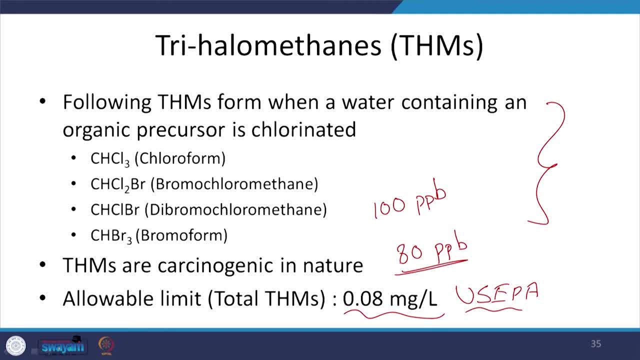 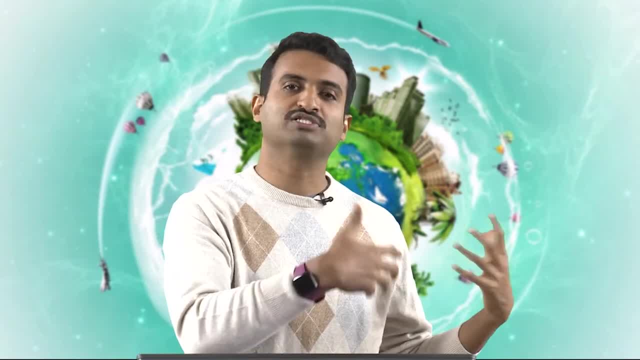 But again, that is because our plants and our standards are still- what do we say? not up to scratch. But you see that we want to improve the quality of life, then obviously we need to look at these aspects too. This is not from the Indian one, I think. this is from US EPA. 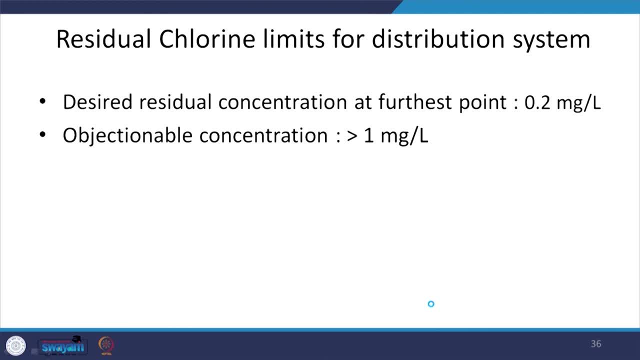 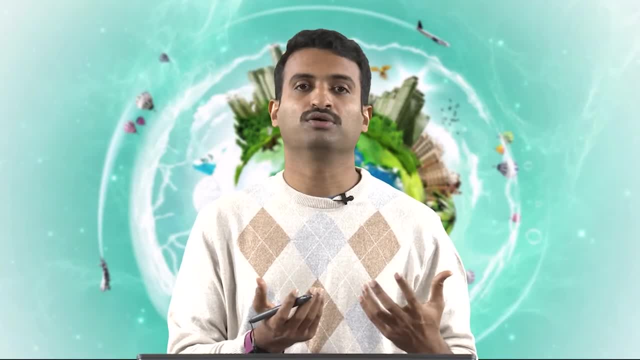 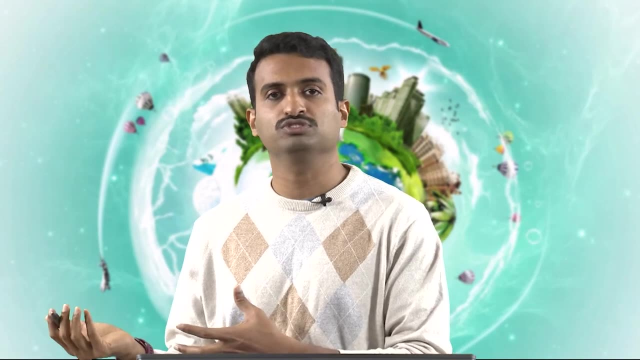 Indian one. we look and look at the relevant standard. So residual chlorine typically. we want that why? because otherwise, if you have pathogen entry, re-entry into the distribution system or entry into the distribution system or microbial growth, you can have issues at the consumer end. So that is why you want to have some residual chlorine even at the furthest point. 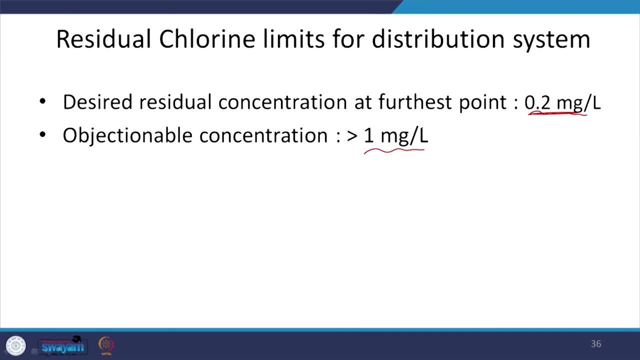 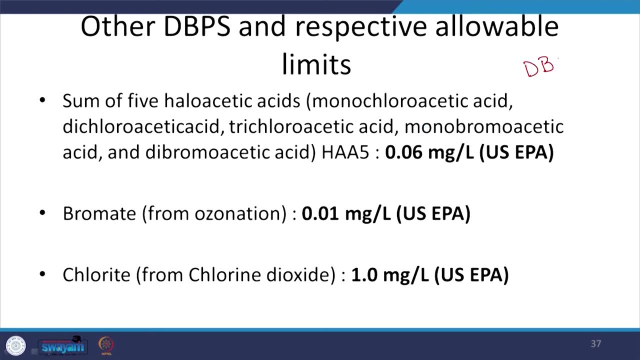 But if it is too high again it is going to be objectionable. obviously, chlorine is a strong oxidizing agent. So there are other- what do we say? other disinfection by-products which are not regulated in India. So there are other disinfection by-products which are not regulated. 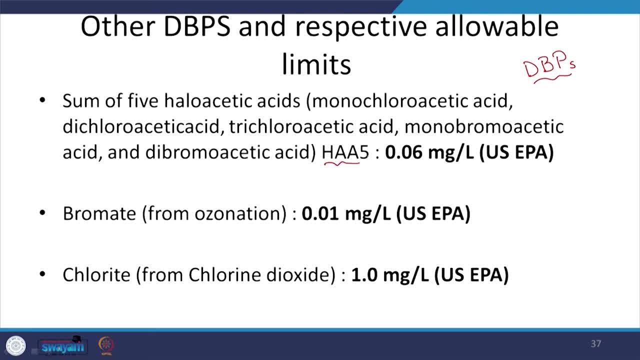 in India. So there are other disinfection by-products which are not regulated in India due to various reasons, But for example, like halo, acetic acid and such, for which in the developed countries we have the relevant standards, but in India we do not have that. So that is. 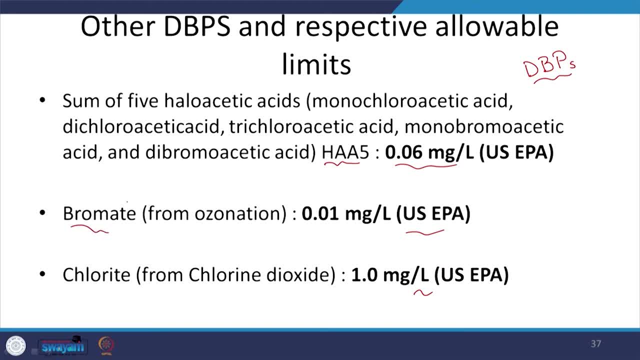 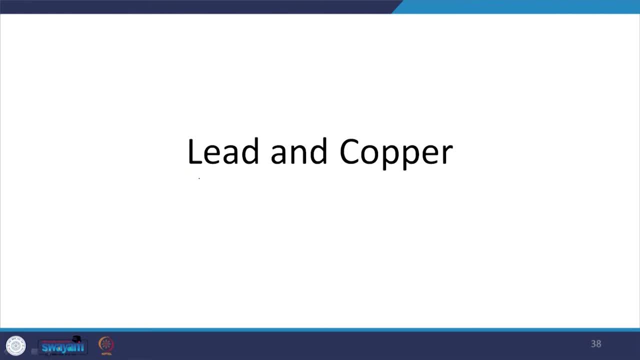 something to keep in mind Again. bromate formed when Br minus reacts with ozone. that is also regulated there. So lead and copper of greater concern in the US because earlier they used to have lead or copper pipelines. So corrosion product of the distribution system typically.